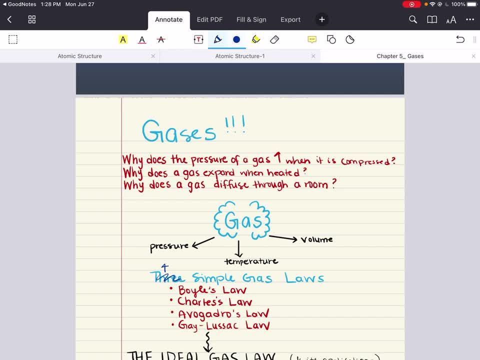 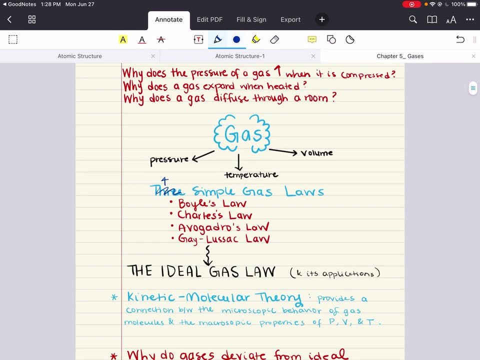 and temperature will allow us to know how to answer questions like why does the pressure of a gas increase when it's compressed? Why does a gas expand when heated? Why does a gas diffuse through a room? In order to answer these kinds of questions, we're going to have to cover topics 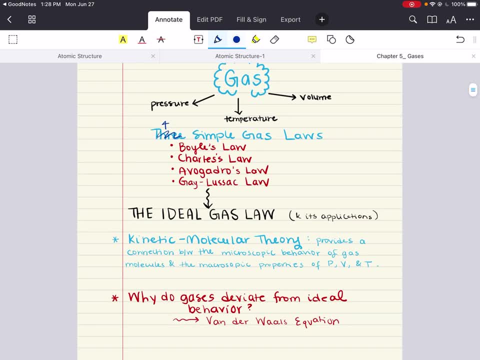 regarding gas laws and everything that you see here on this objective page, We're going to understand the four simple gas laws: Boyle's, Charles, Avogadro's and Gay-Lussac. We're also going to put all those four simple gas laws together to reach the ideal gas law, and even 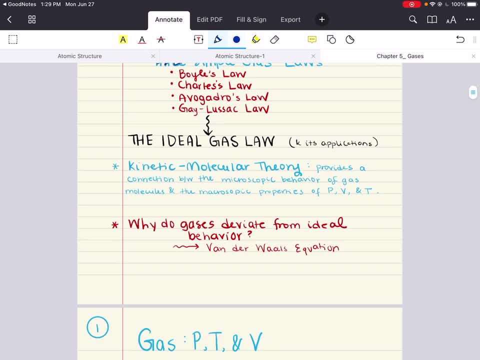 talk about its applications. We're going to cover kinetic molecular theory, which provides a connection between the microscopic behavior of gas molecules and the macroscopic properties of pressure, volume and temperature. We're going to end this chapter by talking about how gases deviate from ideal behavior. This ideal gas law is only applicable when we're talking about ideal. 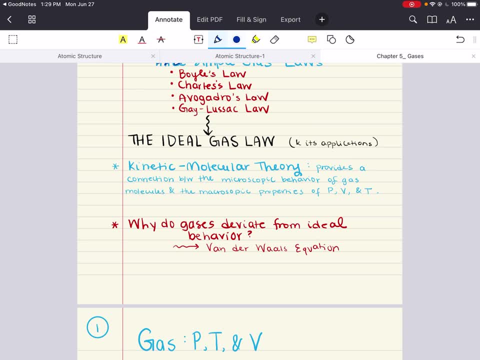 gases, which in the real world that is not the case. What is the correction for that? Although we're not going to get into the details of van der Waals, we're going to talk about the van der Waals equation. It's more of a physical chemistry topic We're still going to touch. 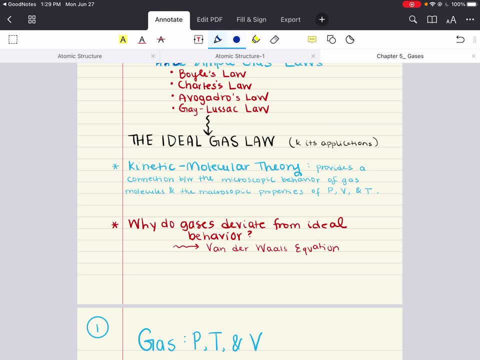 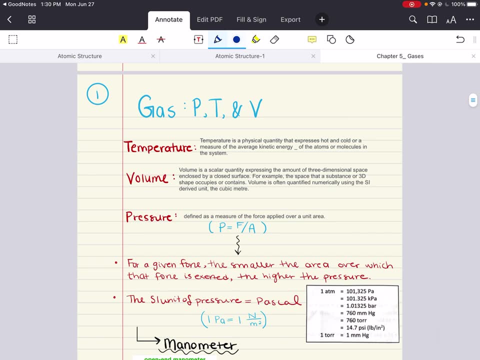 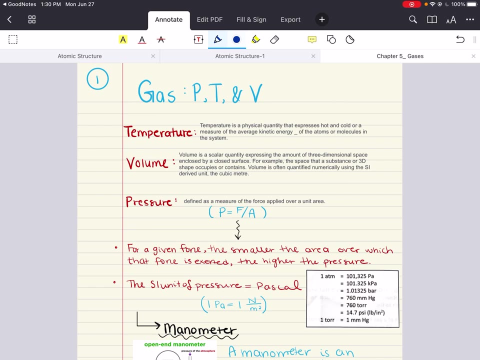 basis on why gases deviate from ideal behavior. Awesome. So let's get started with the first topic and define some important concepts and terminology. Temperature is a physical quantity that expresses hot and cold, or a measure of, if you will, average kinetic energy of atoms, or. 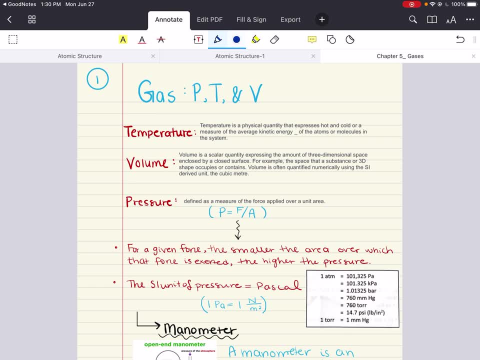 molecules in the system. Volume is a scalar quantity. All right, That expresses the amount of 3D space enclosed by a closed surface And pressure, and this is the most important term that really needs a definition, because you probably have not encountered a. 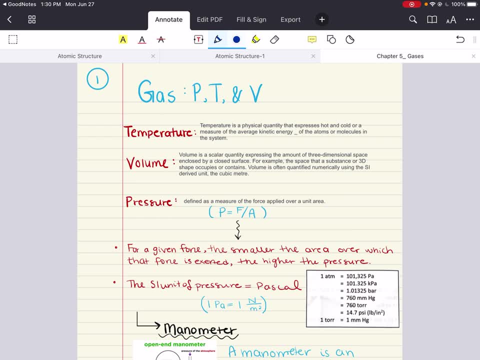 mathematical definition for pressure. It's defined as force per unit area. Every gas exerts pressure on its surrounding, And this definition is defined mathematically as equaling force per area. Now, for a given force, the smaller the area over which that force is exerted, the higher the 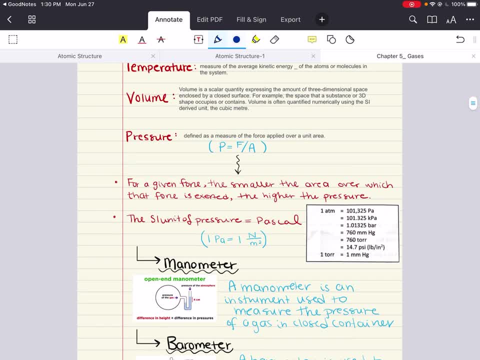 pressure. So now, what are the SI units for pressure? Well, the SI unit for pressure is Pascal, which is also equal to newtons per meter squared. So in other words, one Pascal represents one newton of force exerted over one square meter of area. Now, here in this table, 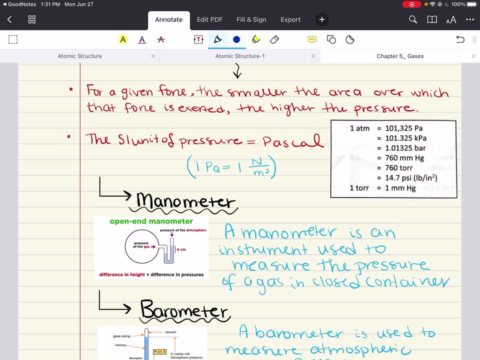 also, what you'll see is some conversions between different units for pressures. These are important to know, especially in problems where you might need to interconvert between different units to answer a problem. So it's good to attempt to commit these to memory. All right Now. 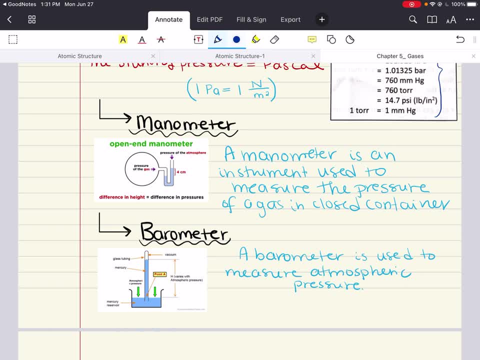 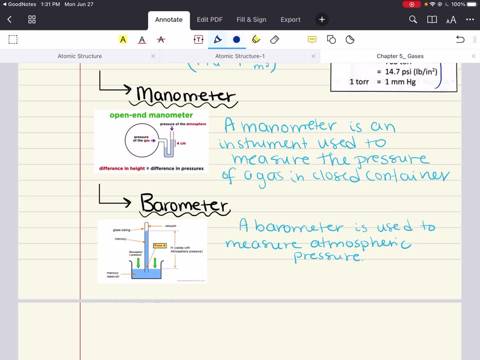 on the topic of pressure. to continue there, there are two instruments that we want to discuss that measure pressure. First one is a manometer. The manometer is an instrument that's going to be used to measure the pressure of a gas in a closed container, And one type of manometer consists of a container. 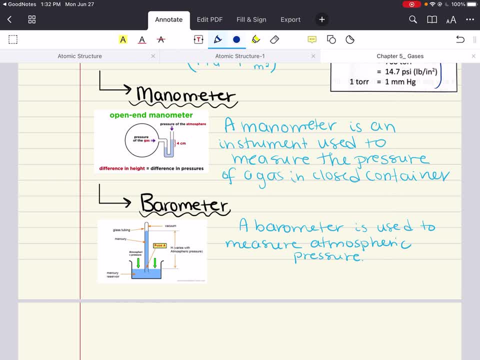 of gas attached to a glass U-tube that's open to the atmosphere, All right. So this tube is partially filled with liquid mercury and the mercury is going to respond to the pressure exerted by a gas in the container on one side and the atmosphere on the. 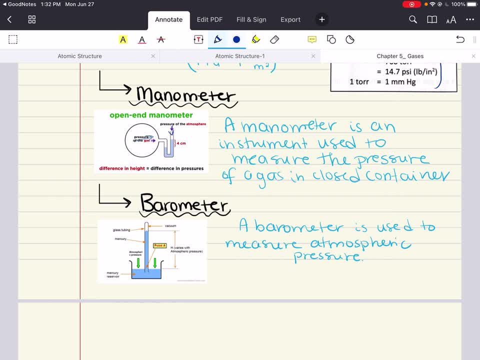 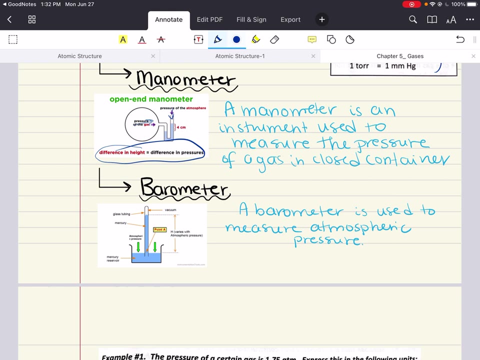 other. So pressure of a gas from one opening, pressure of atmosphere in the other, And the difference in height is equal to the difference in pressure. Now the second instrument that can be used to measure pressure is a barometer. The barometer is used for measuring atmospheric. 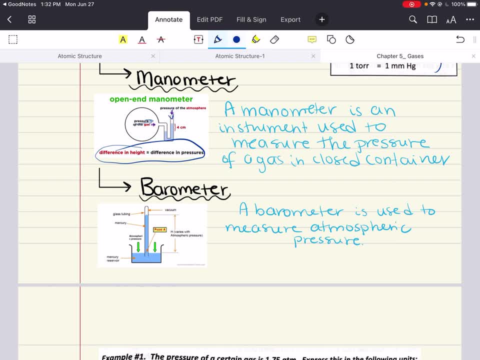 pressure. It consists of a long glass tube that is closed at one end and filled with mercury, And the open end of the tube is covered, inverted and placed in a reservoir Of mercury in a way that prevents air from entering the tube. So then, pressure from the 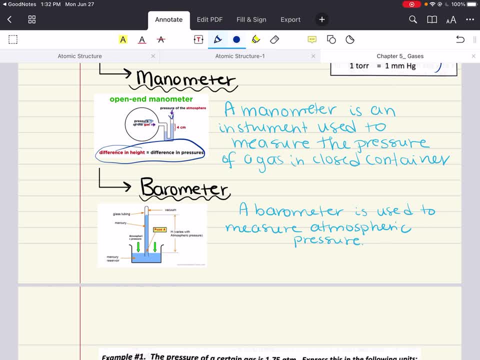 atmosphere is going to press down on the open reservoir of mercury holding mercury inside the tube, And the atmosphere pressure is counted by the pull of gravity on the mercury in the tube And through this difference we can obtain pressure. Fantastic. So, with all that being said, 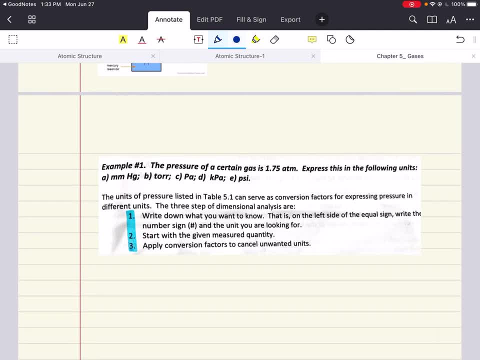 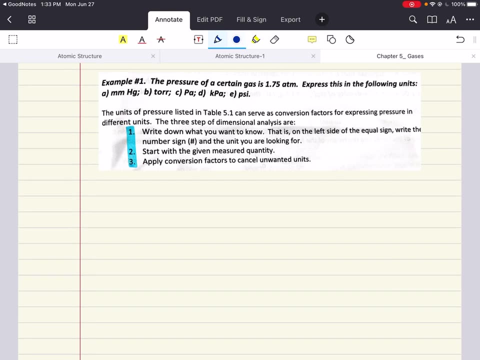 before we jump into the more important topics, we still want to make sure that we are certain how to interconvert between the different units of pressure. So we're just going to pause and do a quick problem on that, All right. This problem says the pressure of a certain gas is 1.75 atm. 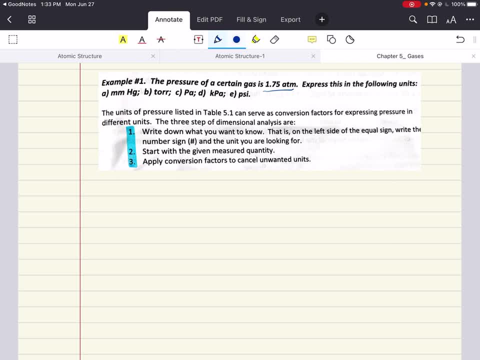 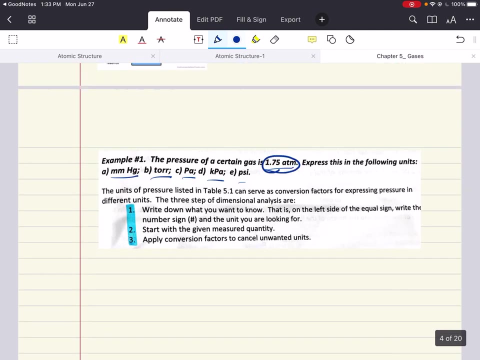 All right. Express this in the following units: MMHE. millimeters of mercury, torr, pascal and sai. All right, So the units of pressure- they're listed here, Okay, And we want to convert this unit of pressure into all the others. All right, So we're going to start off first and 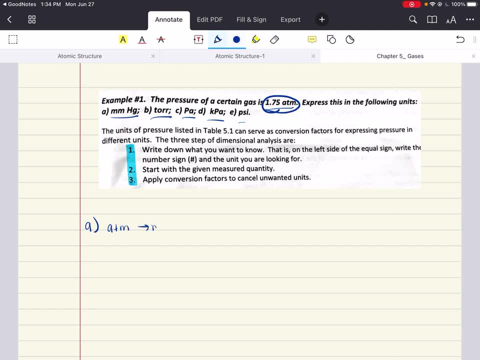 foremost, We're going to go from atm to mmHg, All right. So we're going to start off with what we always know, which is we have 1.75 atm of pressure. We want to convert from this to a milligram of mercury, All right. What's the unit of conversion for this? So we're going to 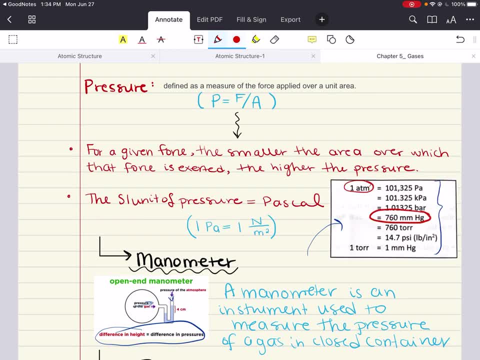 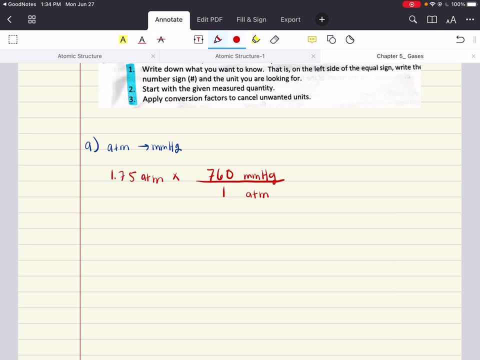 go to our table and we're going to see 1 atm is equal to 760.. So we're going to write that conversion down. That's all it takes. Now, guess what Atm? atm cancels out, and this is the unit. 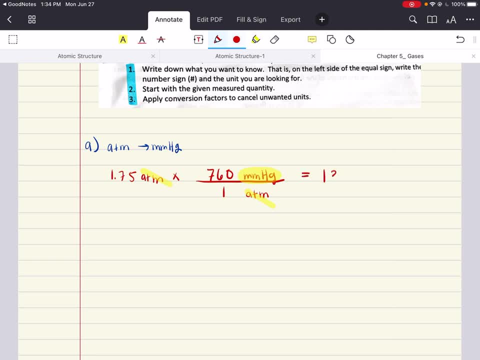 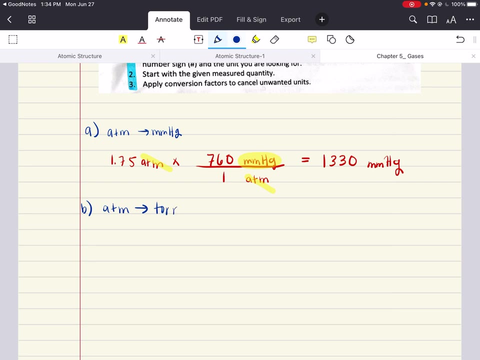 that we're left with. So we plug this into a calculator and what we get is 1,330 mmHg. Fantastic. We just did the first one, All right. Now what else do we need to convert it To? All right. What's the next unit? Tor. All right, We want to go from atm to tor, All right. 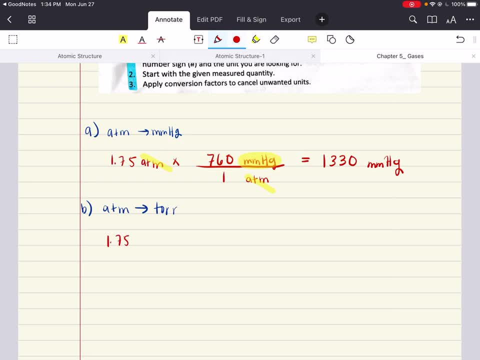 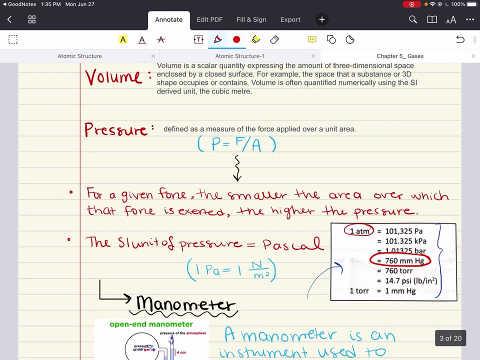 Again, we're going to start off by writing what we already know: 1.75 atm, All right, And we want to go from atm to tor. What's the conversion factor for 1 atm to tor? It's also 760.. Fantastic. 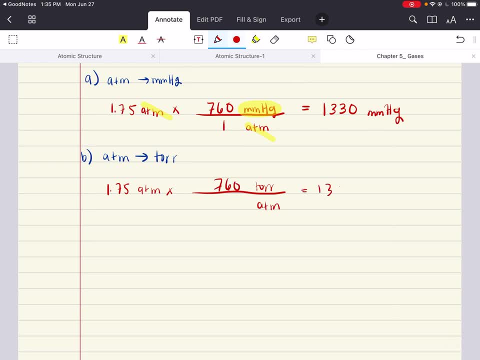 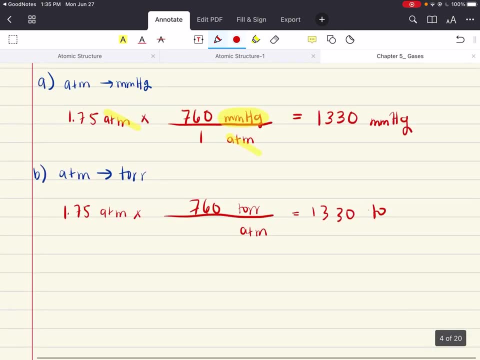 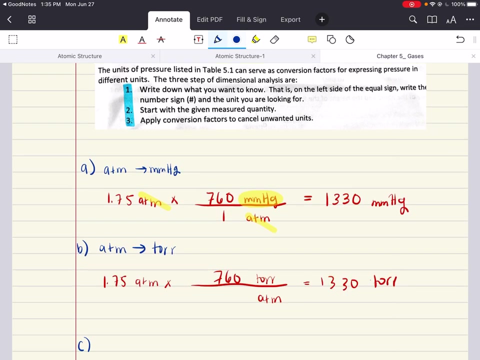 So we'll write that in. All right Again, plug that into a calculator. We're going to get 1,330 tor. Oops, Sorry about that. Tor, Awesome, All right. What is the third unit we want to convert to? All right, Pascal, Awesome. So we're going from atm to pascal. All right, Same thing. 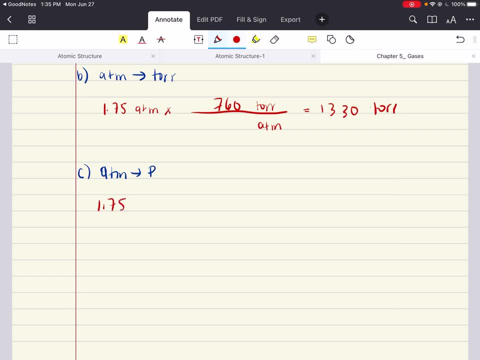 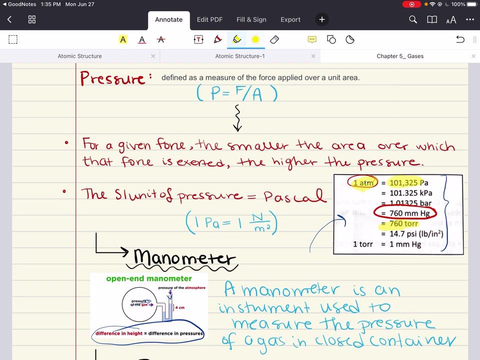 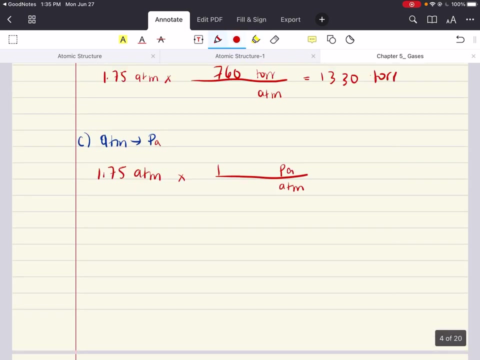 again, We write what we already know. We're starting off with 1.75 atm, All right. And we want to go from this to pascal, All right. Again, we're going to check our table. We want to know what that conversion factor is. 1 atm is 101,325 pascals- All right, Big number, All. 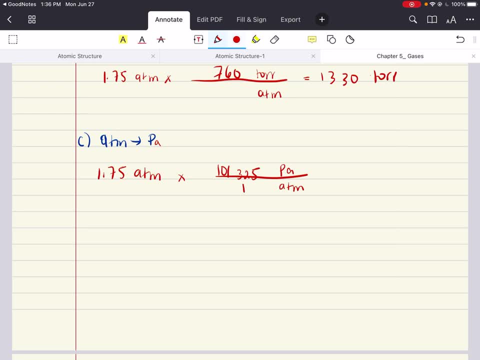 right, So we're going to write that down. Is 1 pascal. Plug this into a calculator: We're going to get 1.77 times 10 to the 5 pascals. Fantastic, Now for kilopascals inside. 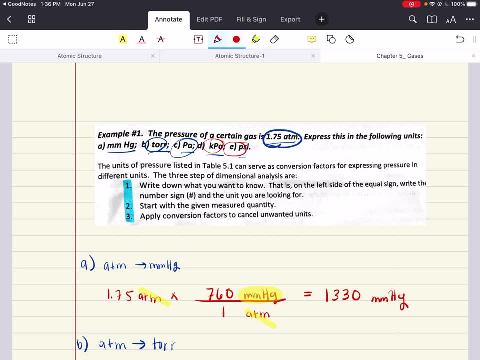 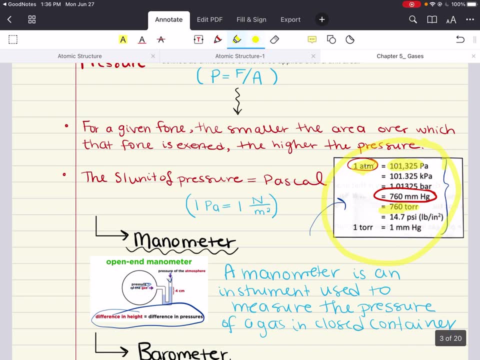 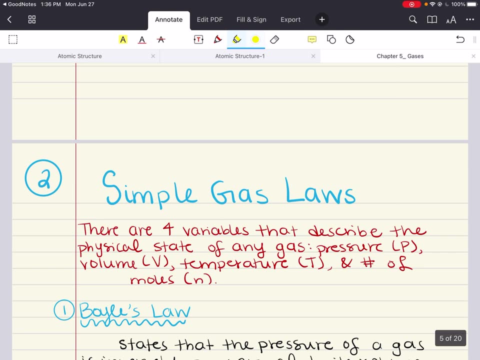 how about you give this a shot and let me know what you get? in the comments below, Same concept. Start off with what you know and use the conversions that you see here to get the unit you desire. Fantastic. Now, with that being said, now that we have defined temperature and 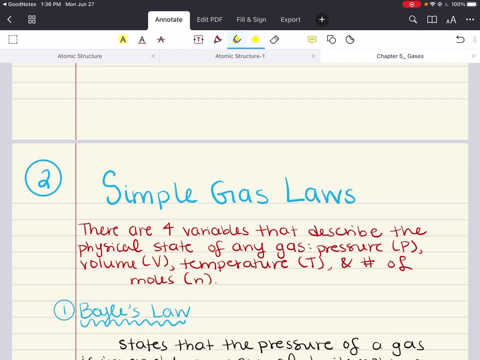 volume and really dived into pressure. we're going to want to discuss now the four simple gas laws. These are Boyle Charles, Avogadro and Gay-Lussac. All right, These are the four simple gas laws And we're going to. 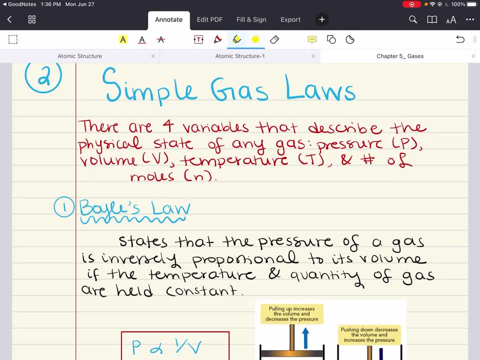 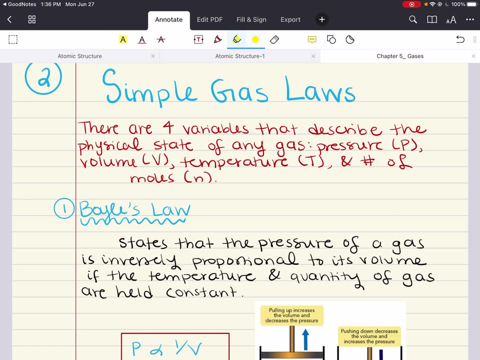 talk about each one specifically. All right, So just to summarize or just to kind of introduce this better, there are four variables that describe the physical state of any gas: pressure, temperature, volume and number of moles. All right, So keep that in mind as we go through. 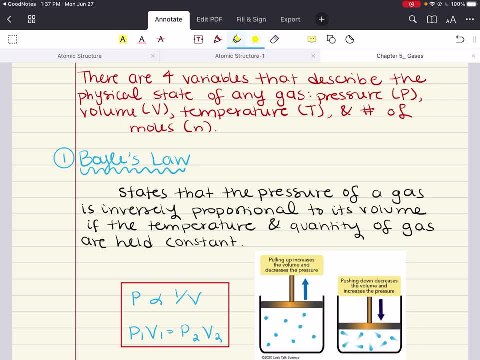 these four simple laws, these four simple gas laws. these gas laws are simply going to relate one physical quantity, one physical state. All right, So these are the four variables that are going to relate one physical quantity to another in some form or another, whether it's to tell you that these two variables are directly proportional. 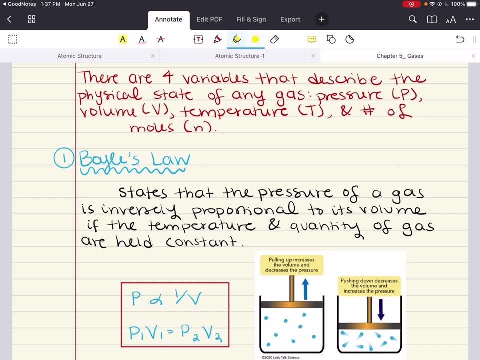 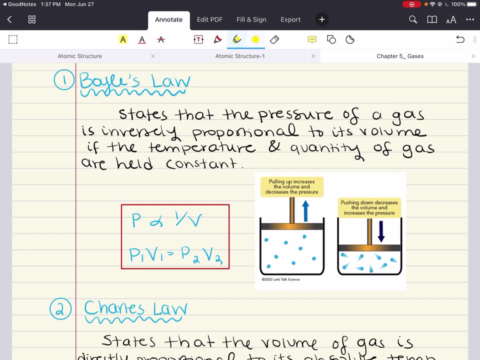 or inversely proportional to one another. All right, It's really going to give us that understanding of how these four variables- volume, temperature, pressure and moles- are related to each other in the sense when we're talking about gases. All right, So the first observation of the 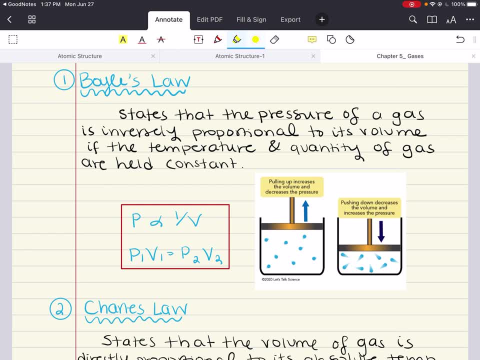 gas law is that the pressure of a gas is inversely proportional to its volume. if the temperature and moles are held constant, All right. We can easily express this: Temperature and moles are held constant. When they are held constant, we can say the pressure is inversely proportional to the 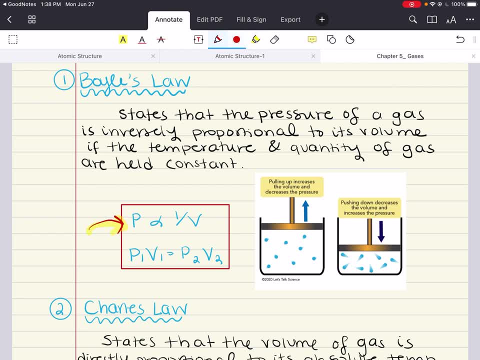 volume. This is what this expression describes. Pressure is inversely proportional to volume, All right. So as volume increases, for example, pressure decreases, All right. As pressure increases, volume decreases. This is what that means when we say inversely proportional. 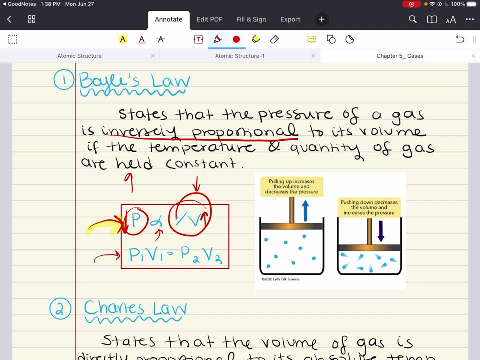 All right. We can also write this. when we're relating two states, All right. When we're relating the pressure and volume of one state to another, All right. Since they're inversely proportional, we can write this mathematical expression: The pressure P1 times V1 is going. 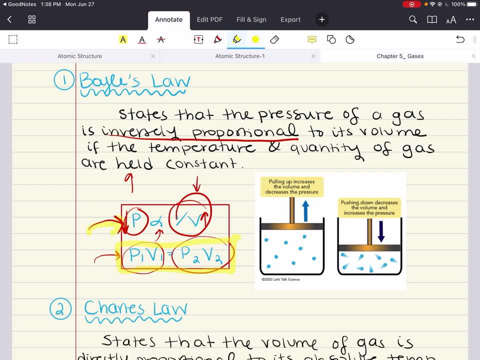 to equal P2- V2.. All right, So we can write this mathematical expression: The pressure P1 times V1 is going to equal P2- V2, where 1 is state 1 and 2 is state 2.. All right, So another way to visualize. 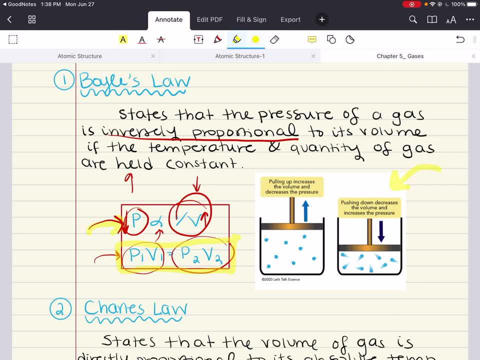 this relationship is in this diagram right here. All right, Pulling up increases the volume, All right, Which means that's going to decrease the pressure. Or if you decide to pull this down and you decrease the volume, guess what? The pressure is going to increase. And that's partially because 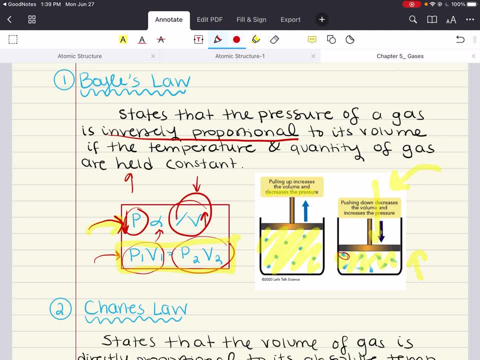 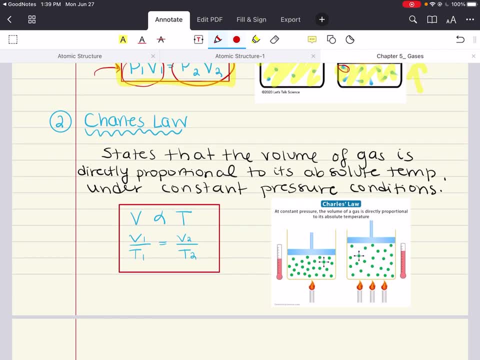 now you have more things interacting with the walls at a faster rate And that's going to increase that pressure when you decrease that volume. all right, Charles' Law. Charles' Law states that the volume of a gas is directly proportional to its absolute temperature under constant pressure. 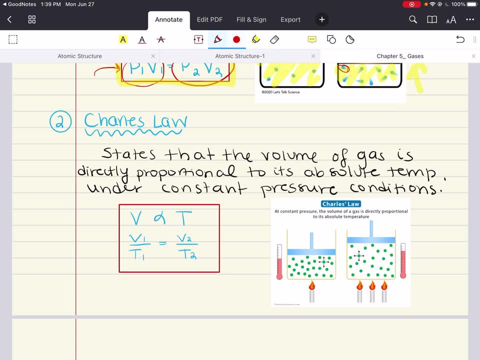 conditions. So when pressure is constant, all right, then volume is directly proportional to temperature. all right, directly proportional. That's what this mathematical expression relays, all right. And that means if we're trying to write, if we're trying to compare the volume, 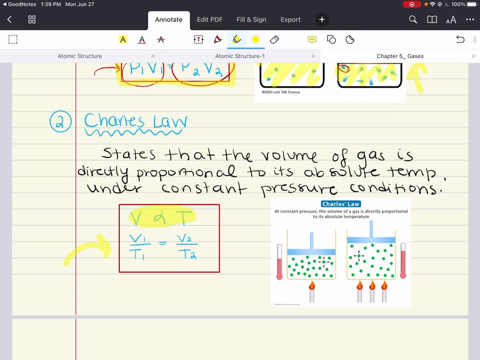 and temperature of state one to changes to state two. we can write an expression where V1 over T1 is going to equal V2 over T2, all right, where one relates to state one and two relates to state two, all right. So in essence, at constant. 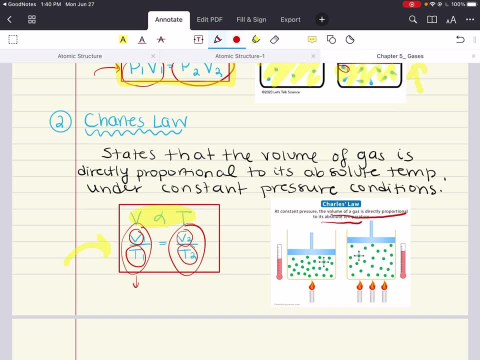 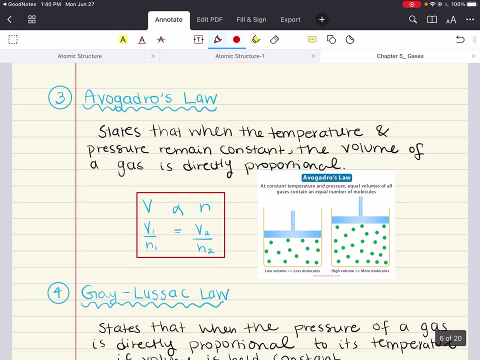 the volume of a gas is directly proportional to its absolute temperature. Fantastic. Now Avogadro's Law. all right, this is the third law- states that when the temperature and pressure remain constant, the volume of a gas is directly proportional to the number of moles of gas. 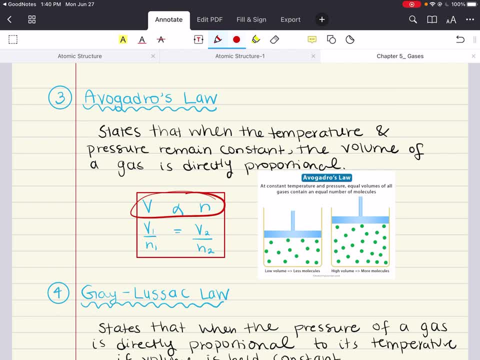 all right, So volume is proportional to the number of moles. This is what this expression. all right, So volume is proportional to the number of moles of gas. And again we can write: when relaying two states, V1 over N1 equals V2 over N2,. all right, At constant. 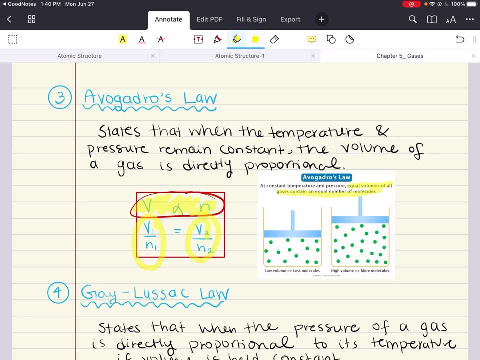 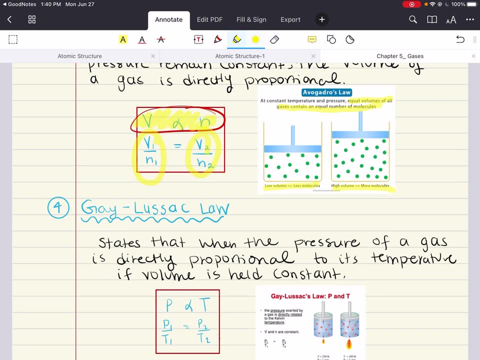 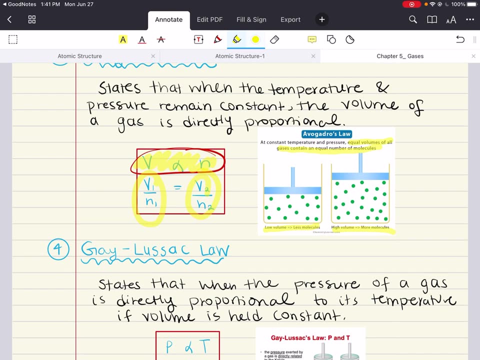 temperature and pressure. equal volumes of all gases contain an equal number of molecules: Low volume, low molecules. High volume, more molecules. all right, Simple as that. Now there are two important consequences of Avogadro's Law. First, when solving gas stoichiometry problems. 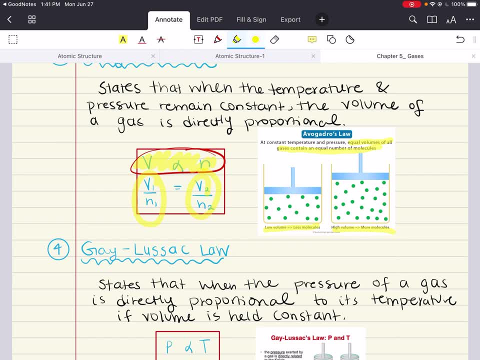 all the gases are measured at the same temperature and pressure. So instead of using mole to mole ratio, we can use liter to liter ratios. all right, And we're going to elaborate more on this when we get to some practice problems. The second important consequence of Avogadro's Law is that the 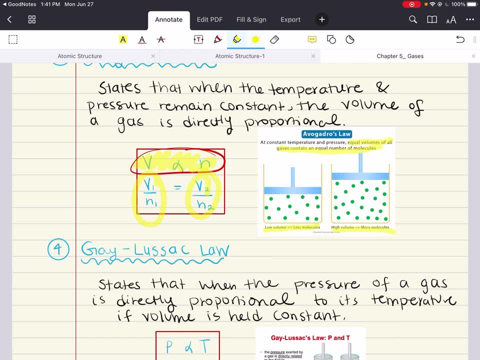 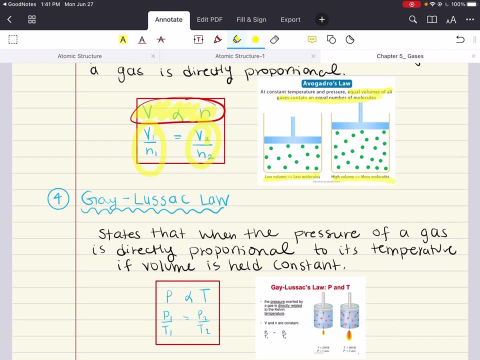 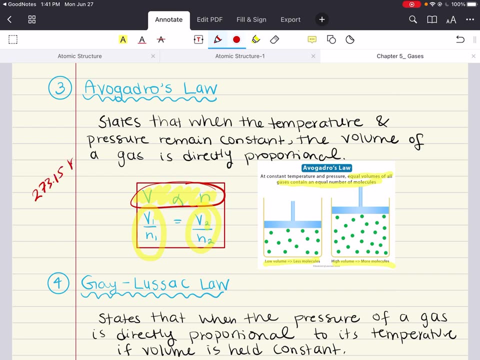 molar volume of any gas at standard temperature and pressure, all right, is 22.4 liters. Now two things. What does STP mean, or what does standard temperature and pressure mean? It means that we're operating at 273.15 Kelvin and at 1 ATM. all right, This is referred to as 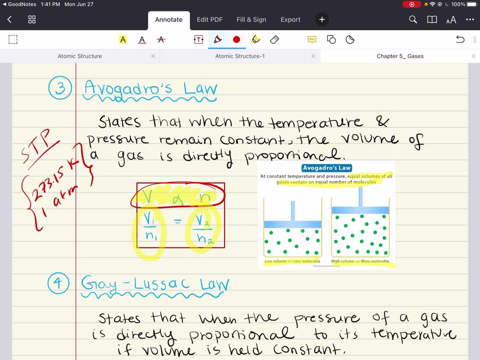 standard temperature and pressure conditions. When you are operating under a standard temperature and pressure conditions, the molar volume of any gas is equal to 22.4 liters. That's an important number to keep in mind, all right, And this is the number we might use when we're using liter to liter ratios. 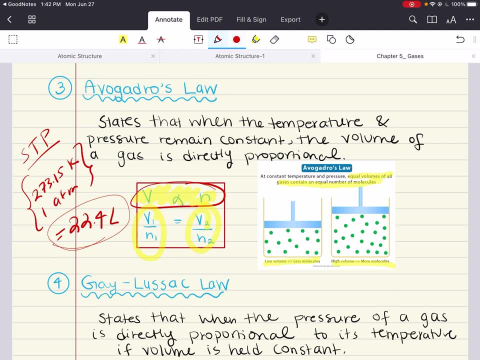 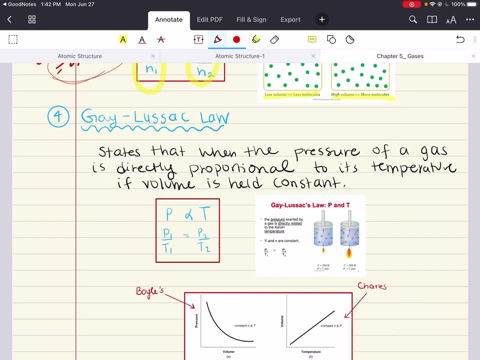 when we're working with gases, Awesome. The fourth law is the Gay-Lussac Law. I'm so sorry I might not be pronouncing that right, especially the second name. I think it's Lussac but I'm not 100% sure. But anyways, this law states that when the pressure of a gas 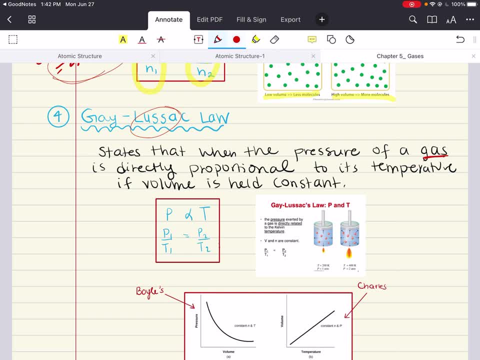 is directly proportional to its temperature. I'm sorry states that when the pressure of a gas is directly proportional to its temperature. I'm sorry states that when the pressure of a gas is directly proportional to its temperature, if a volume is held constant, So then we can write. 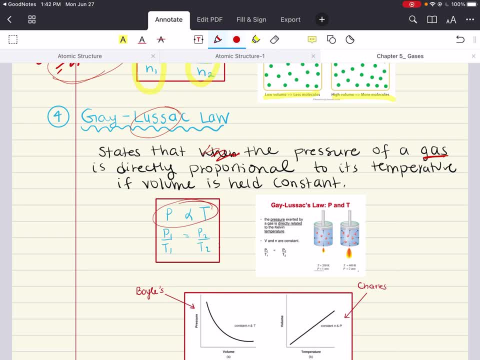 this relationship. Pressure is directly proportional to temperature And if we're relaying two states, then we can write: P1 over T1 equals P2 over T2, all right. So the pressure exerted by a gas is directly related to the temperature And you can see that in this. 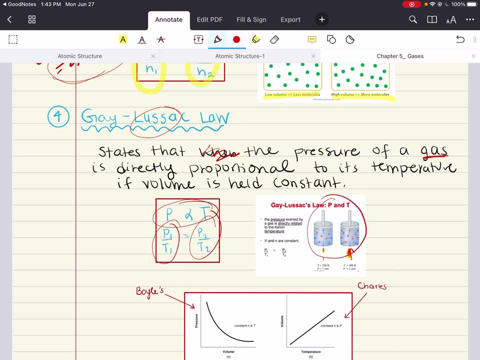 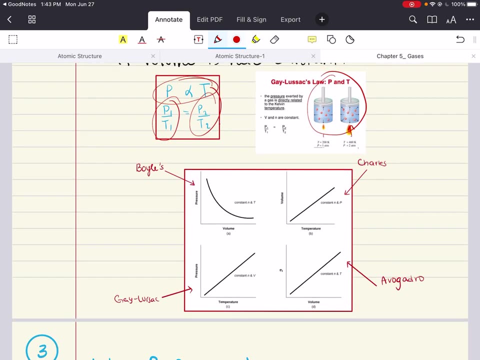 diagram here. all right, As you increase temperature, all right, you're increasing pressure. You have more collisions to the wall of the container. The gases collide with the walls more, increasing pressure. that way, all right. And here at the end, we have a graph to demonstrate. 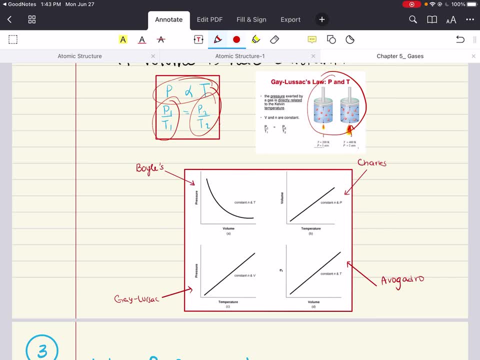 these relationships of the four simple gas laws. right, With Boyle's Law, we said that pressure and volume are inversely proportional. all right, And this graph demonstrates that. all right. Avogadro's Law says that volume and temperature are directly proportional. all right, And this? 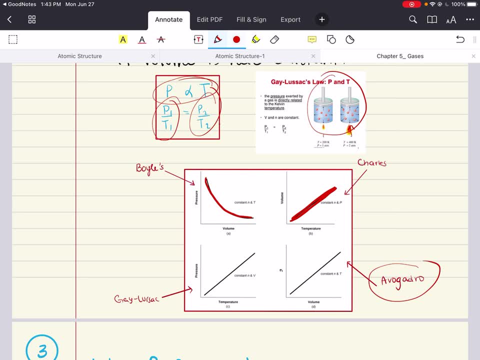 graph demonstrates that. all right, Avogadro's Law says volume and moles are directly proportional. all right, This diagram, this graph, demonstrates that. And the Gay-Lussac Law states that temperature and pressure are directly proportional. all right, And this demonstrates that. 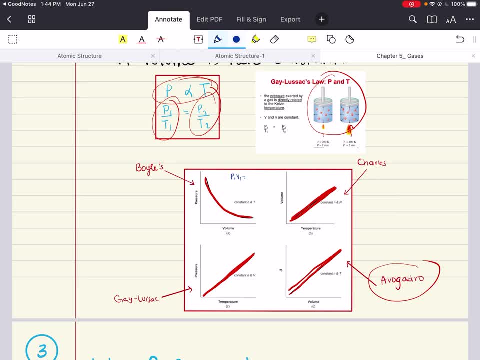 And what helps is always to write. you know even the equations for each one of these, Just to have it all concise in one place, all right. So these are important to remember And we're actually going to do something really cool with all these relationships, And that's kind of. 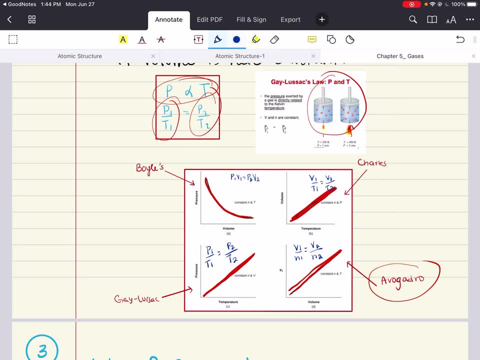 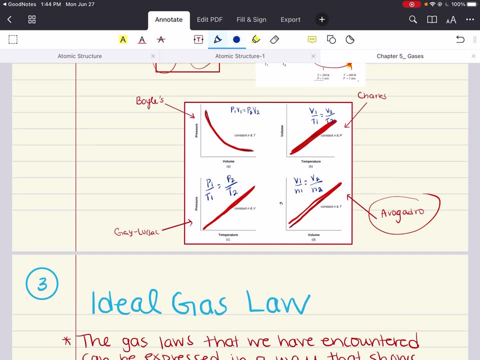 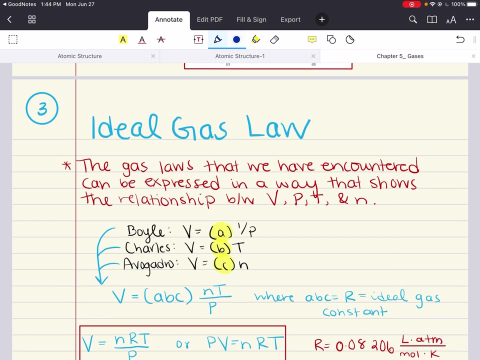 put them together to get at a one-form ideal gas law. all right, So this was all background information that's going to let us segue into the ideal gas law And it's application. So the four gas laws that we have encountered can be expressed in a way. 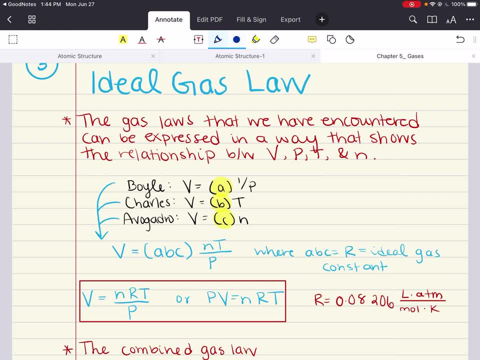 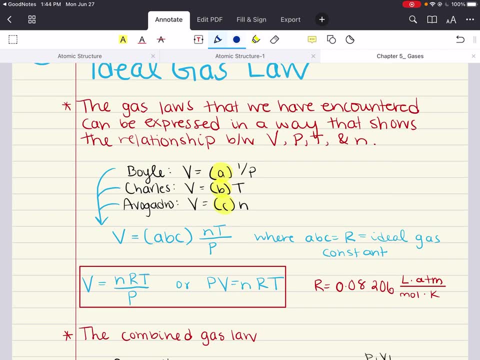 that shows the relationship between volume, on one hand, and pressure, temperature and number of moles on the other. all right, So this is just an attempt to try to reach a single formula that puts all of this together. So what we're going to do, in order to do that, is we're going to write. 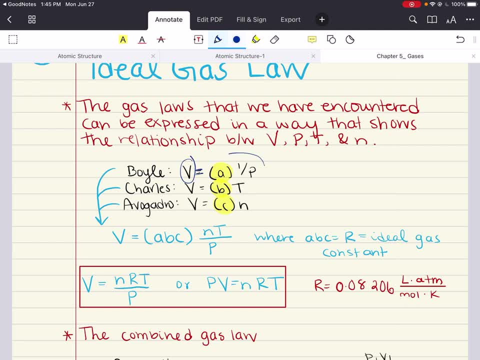 volume on one side and we're going to relay it to something else. So for Boyle's Law he said volume was related to pressure inversely. so So we write V, all right. equals 1 over P times some constant. that's going to allow this relationship to happen, all right. 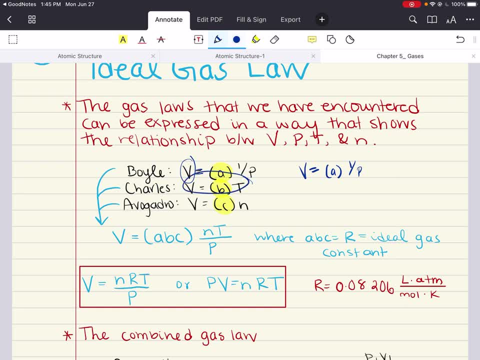 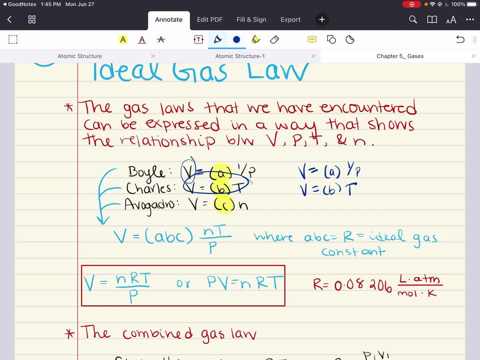 Same thing with Charles, right, We related volume to temperature. So we write: V is going to be equal to temperature, you know, and that's manipulated by some constant to make this true Avogadro. we related volume to moles. all right, We're going to say some constant. 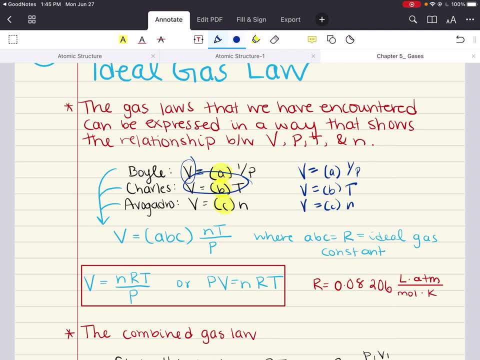 that we can multiply moles by will allow this relationship to happen. So we're going to say to be true, all right, So we're just mathematically dealing with these so that we can go ahead and write one expression that puts all these variables together. all right, So we have these three. 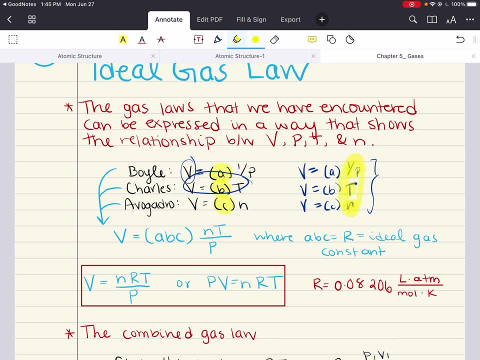 expressions of volume. all right, So we're going to take all of these three variables and we're going to put them together. We're going to put them together where volume is equal to moles times temperature over pressure, just like we've expressed it individually here. all right? 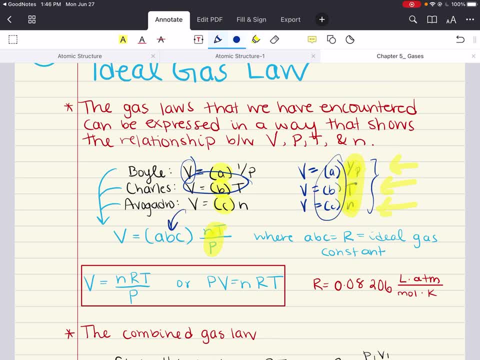 Now A times B times C, we can put it here, but essentially those are just constants. So we can redefine ABC to just equal R, which is the ideal gas constant. all right, And actually this has a specific value This constant has. we know what this constant is. all right, And this is the. 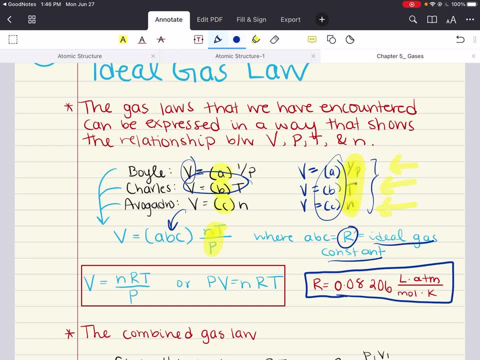 constant right here. This is very important for you to remember. We will be using it in a lot of practice problems that you know that revolve around the ideal gas law. So now by expressing volume. all right, expressing volume as it relates to pressure, and then temperature and the number. 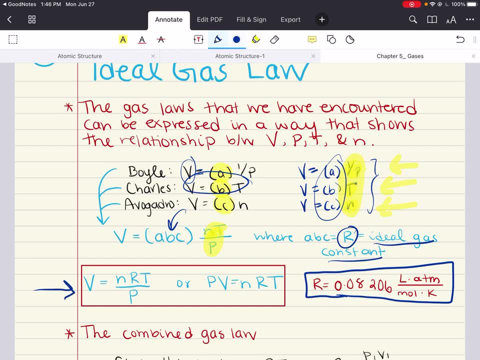 of moles and putting it all together, we've reached this formula that relates and shows the relationship between volume, temperature, pressure and moles, And this is our ideal gas law. Volume is equal to moles times temperature times our gas constant. 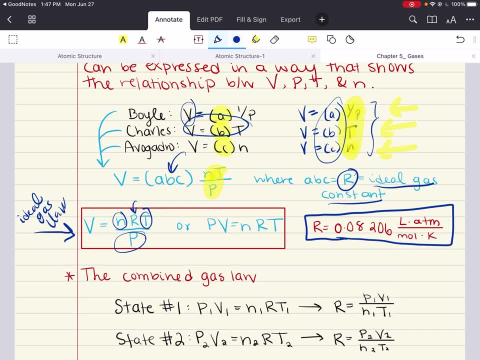 over pressure. all right, Fantastic. Now we can also use the ideal gas law to determine how our variables- temperature, pressure, volume moles change, going from state one to state two. all right, One problem that we encounter involves a gas undergoing changes in its conditions. 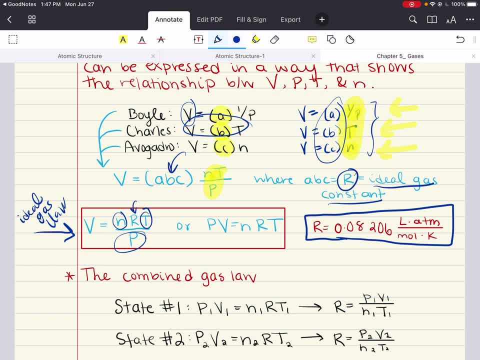 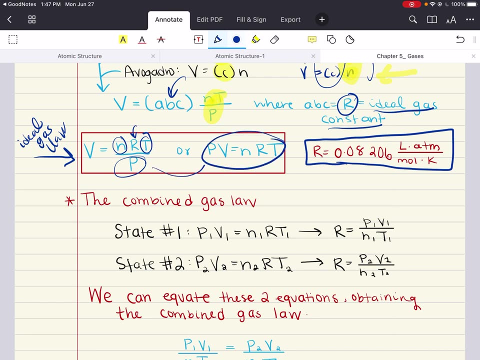 and we can use equating the two ideal gas expressions for each state to obtain what is called the combined gas law, to say to solve for our variables. all right. So, for example, all right, here's our ideal gas law. all right, There's two ways of writing it. It's the same thing. We just moved pressure over to. 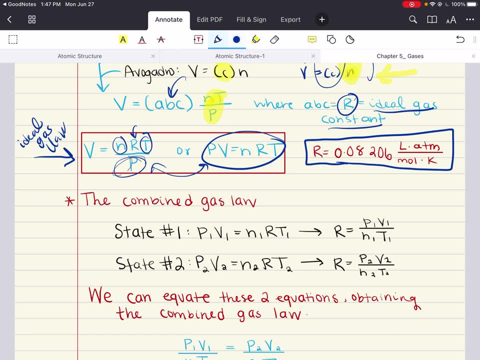 one side all right. Let's say we're in state one, whatever state one is all right, And we can express state one as being: P1V1 equals N1T1 times P1V1. equals N1T1 times P1V1. equals N1T1 times P1V1. 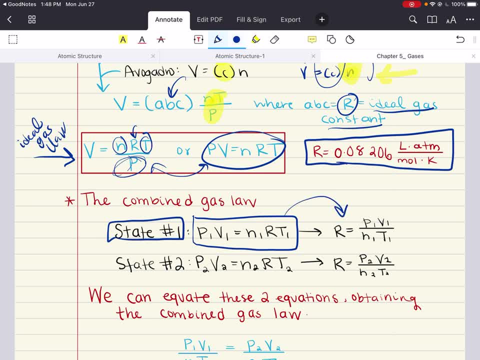 times the gas constant. We can rearrange this to solve just for R. How do we do that? Well, we're going to divide by N1T1 on both sides, all right. On one side, all these cancel out and what we get is R equals P1V1 over N1T1.. Now imagine we're in state two. all right. 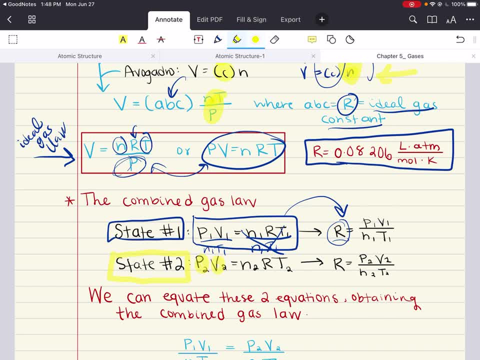 of a gas. We can express this new state as: P2V2 equals N2T2 times our gas constant. all right. Now again, we want to redefine, We want to move these variables so we can redefine R in state two. all right, R is just a constant. So what we're going to do here is we're going. 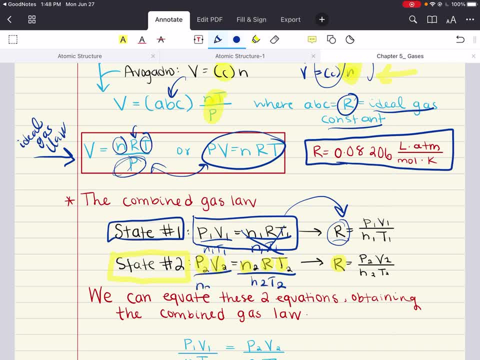 to divide by N2 and T2 on both sides. all right, These cancel out, and now we can write: R equals P2V2 over N2T2 for state two. So now we have our state, one expression, and we have our state. 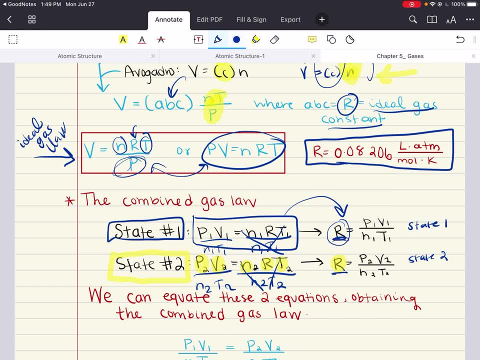 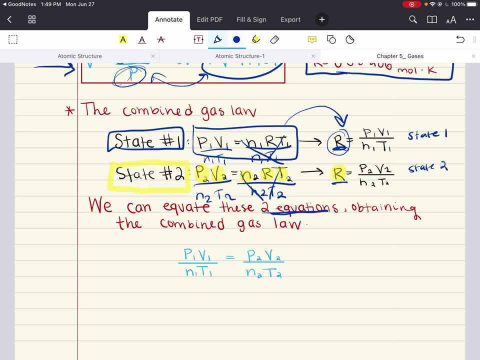 two expression. They both equal R, and R is just a constant. So guess what we can do now? Now we can equate these two equations and obtain the combined gas law where we have P1V1 over N1T1 equals P2V2 over N2T2, and now we have a way of equating two. 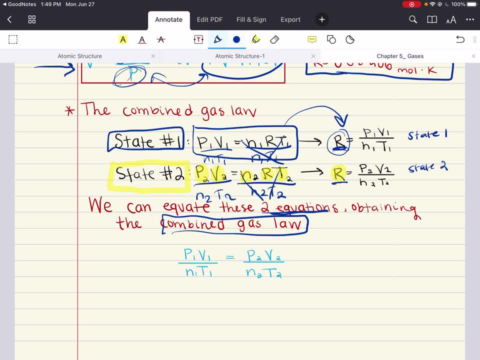 ideal gas expressions for two states, for two different states to solve, for variables. all right, Now, before we jump into some practice problems, we're going to do a little bit of for gas laws that we have discussed and seen so far. There's one more thing we want to do. 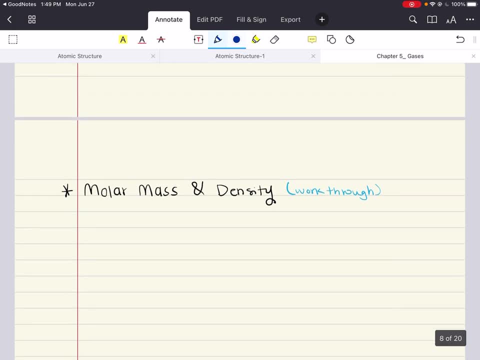 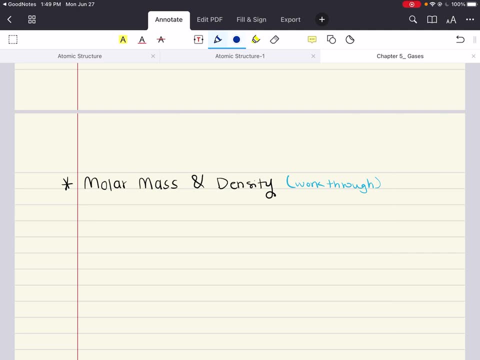 and that's derive an equation where we can write the ideal gas law in terms of molar mass and density. all right, This is going to be important to solve certain problems as well, to have this relationship, all right. So let's define a way, Let's find a way to define our ideal gas law. 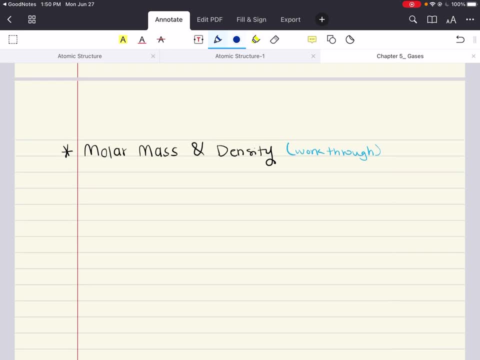 in terms of molar mass and density. So far we've seen our ideal gas law in terms of four specific variables: pressure, volume, moles and temperature. We can re-express this to have molar mass and density so that we can obtain and evaluate variables about our gas. 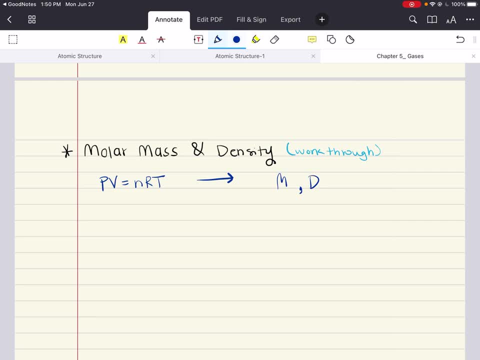 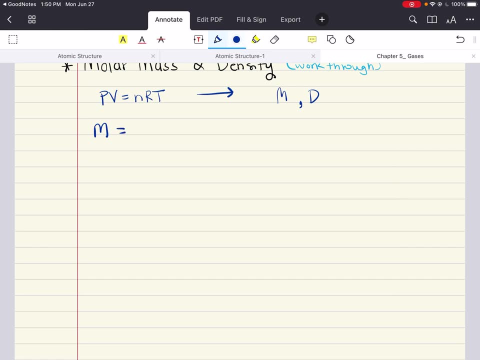 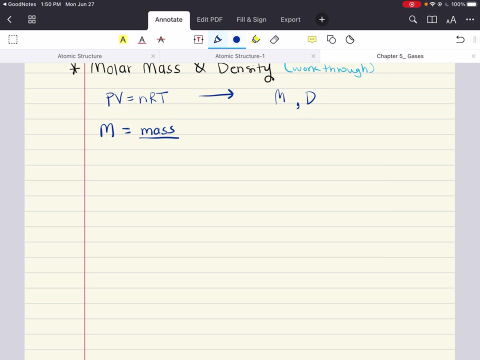 if we only have molar mass and density to work with, all right. So let's do this From the start. what was molar mass defined as Well? if you saw my chapter three videos define molar mass as mass over moles. all right, Over moles. all right, This was our. 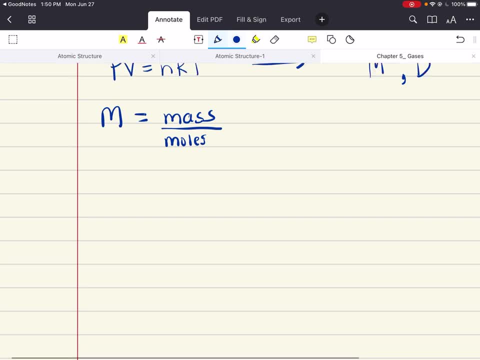 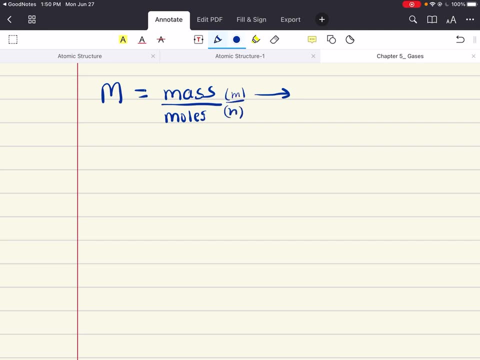 definition of molar mass. okay, We're going to rearrange this. all right, This is m over n. all right, Just thinking about it like that. all right, We're going to rearrange this so that we have an expression for moles n. all right, We can multiply this over here and then divide by. 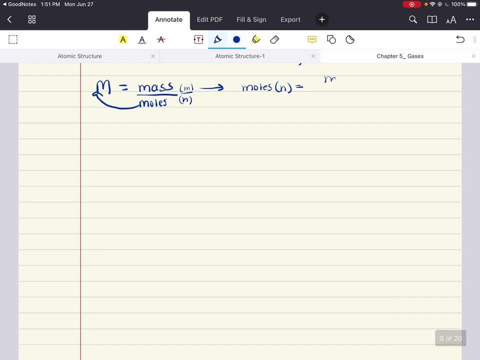 mass, And so we can get a definition for moles that's actually just mass over molarity, all right, Fantastic. Now we're going to take our ideal gas law: PV equals nRT, all right. And we're going to take our new expression of n of moles, and we're going to 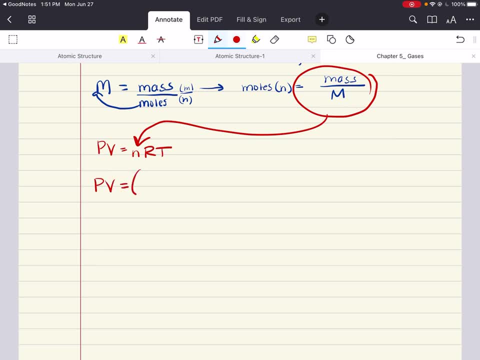 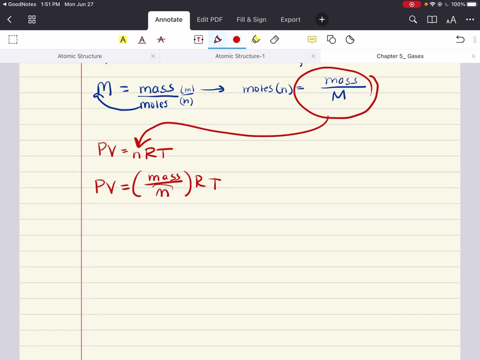 plug this in here. What do we get? We get PV equals mass over molar mass, RT. all right, Fantastic. Now something else we're going to do here is rearrange so that we can solve for m for molar mass. all right, So we're going to rearrange, That means we're going to move m over. 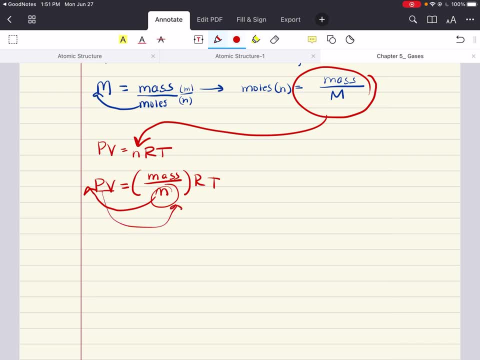 here, and then we're going to divide by PV over here, And what do we get? Well, we get- and I'm going to write this in a different color- we get molar mass equals mass over volume. all right, Because we've divided by volume times RT divided by. 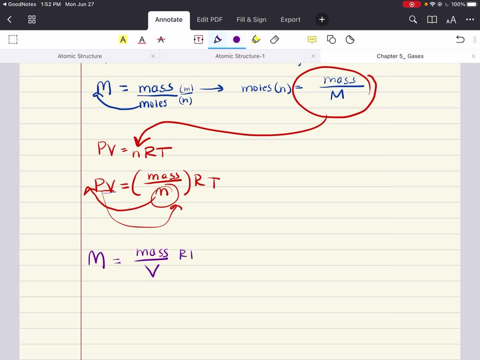 sorry, RT divided by P. all right, So we get something like this Now. we talked about this in chapter one, but you may have forgotten and that's okay. There is a term that's defined as mass over volume. all right, If you remember from chapter one. 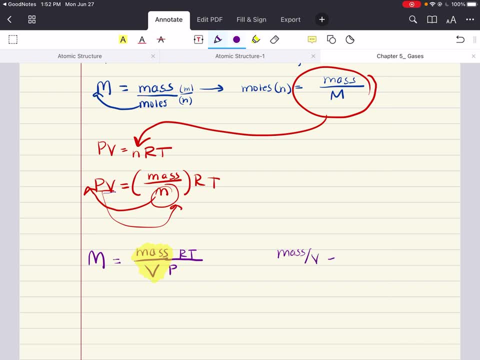 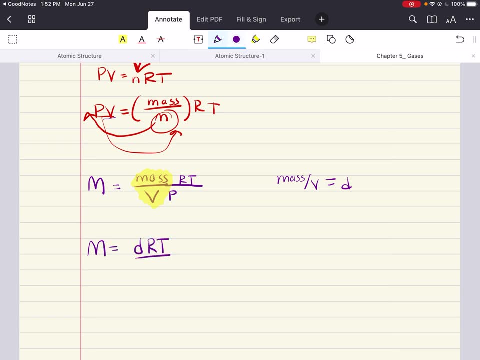 mass over volume is equal to density, all right, And so now we can rewrite our final version of molar mass as density Times, RT over P, all right, So this is an expression that is going to serve us in answering certain problems that relate to the ideal gas law and combined gas law. Having this relationship is: 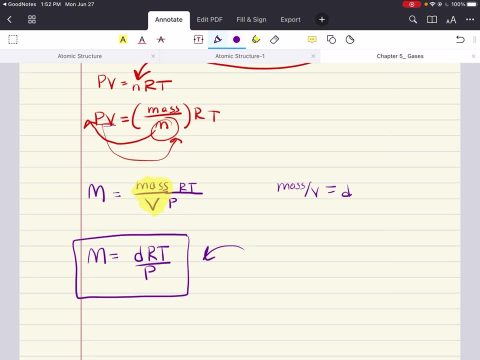 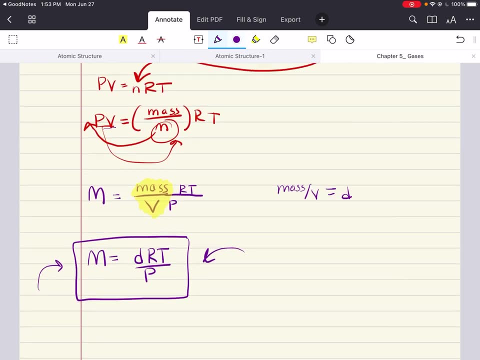 going to be important in the coming chapters. So since we've discussed how to obtain this, now, all right, we've kind of derived it. all right, It's important that you commit it to memory, and we're going to do some. 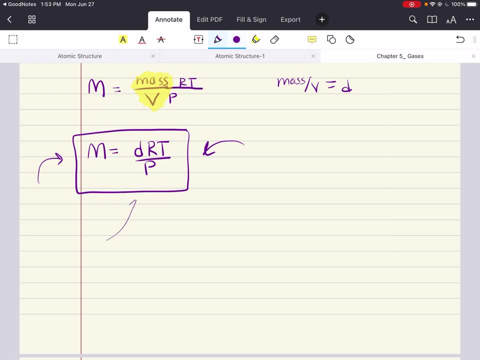 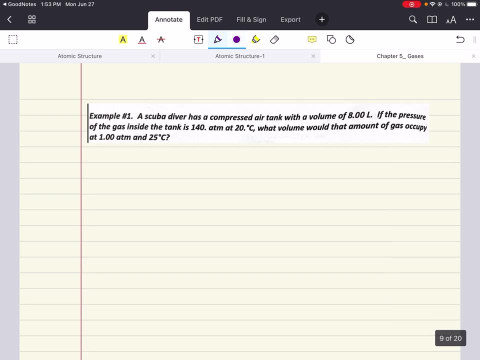 practice problems and we're going to encounter why this relationship is important in this chapter and in the coming chapters. all right, So now that we've discussed this, let's jump into some practice problems. all right. This first problem says a scuba diver has a compressed air tank. 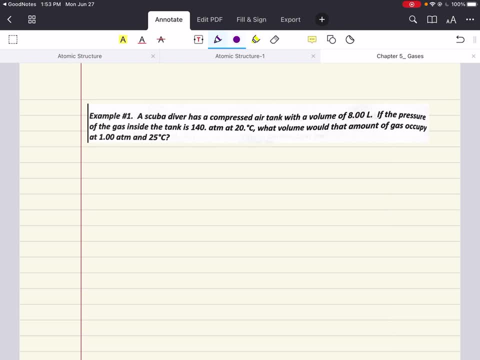 with a volume of eight liters. If the pressure of the gas inside the tank is 140 atmosphere at 20 degrees Celsius, what volume would that amount of gas occupy At one ATM at 25 degrees Celsius? all right, So we have this kind of scenario set up for us. 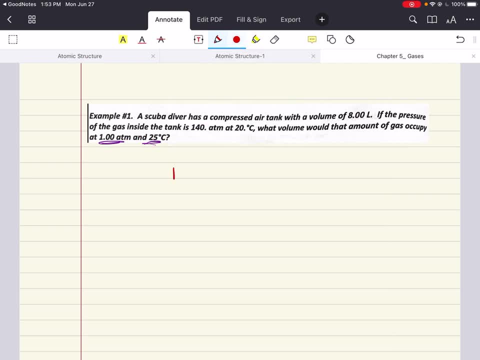 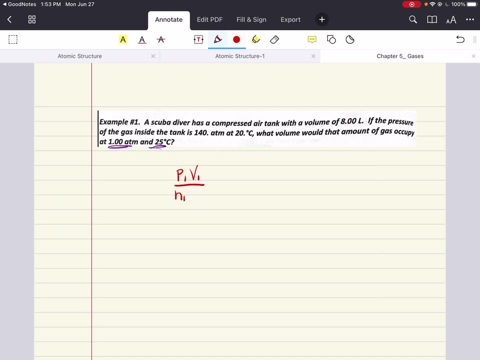 before and after scenario. all right, And so obviously we're going to have to use our combined gas law. all right, We're going to have to use our combined gas law to relate things in one state to another, all right, So we're going to write our combined gas law here, P1 V1 over N1 T1. 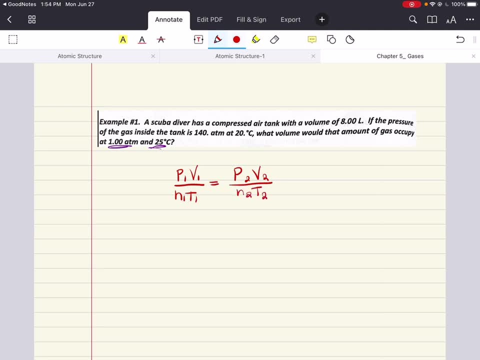 equals P2, V2 over N1, T1.. All right, We can tell that we need to use this because a scuba this problem says: if the pressure of the gas tank is this at this degree, what volume would it be at this new? 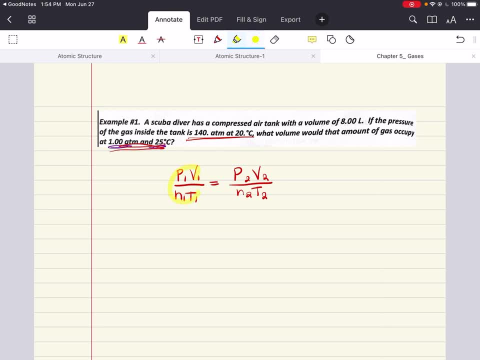 pressure and temperature, So we can tell we're relating one state to another, sort of like a before and after, if you will. if that helps you think about it. all right, So let's write down what we know about state one. 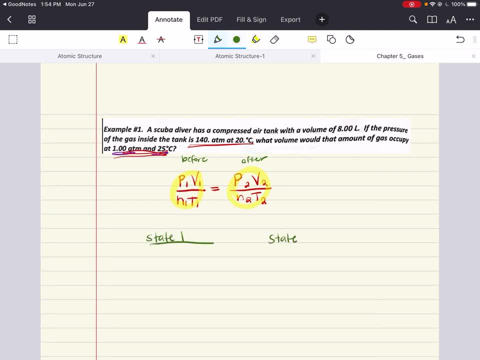 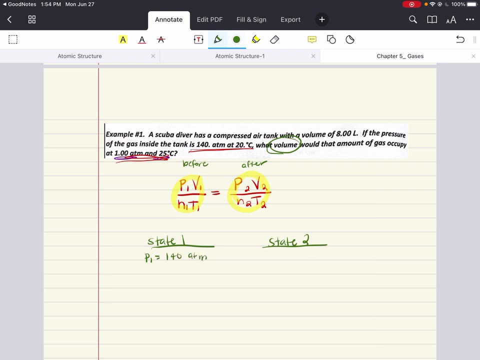 P1 versus what we know about state two, And that way we can figure out how to rearrange this to solve for the volume: all right, The V2,, if you will. All right for state one. we know what P1 is. all right, It's 140 ATM, All right, that's what it says, right here. 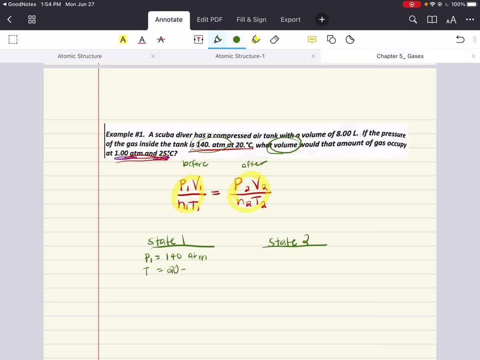 We also know the temperature. The temperature is 20 degrees Celsius. but remember, for ideal gas law, you always want to work with Kelvin. To get from Celsius to Kelvin, you simply add what you have in Celsius. You simply add what you have in Celsius and you get what you have in Kelvin. 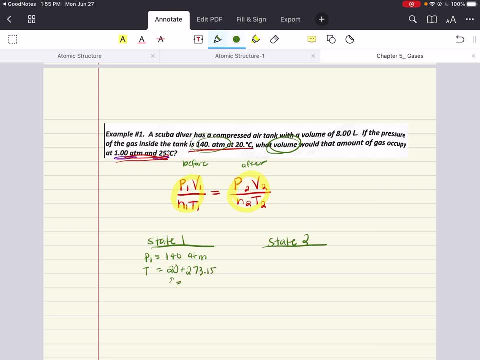 Plus 273.15. And so we get 293 Kelvin. Always want to work in Kelvins for ideal gas law. All right, fantastic. We also have volume one. It's right here. eight liters, all right Now. 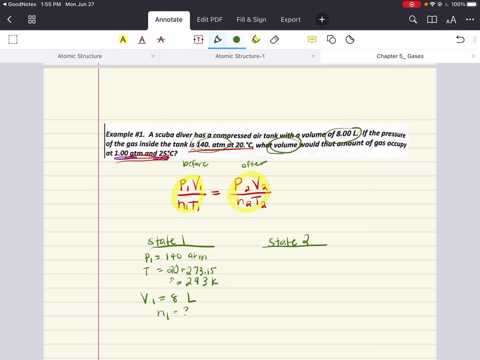 N1 is not given. We don't know it. If you look at state two, we also don't know what N2 is. all right, So we don't know what N1 or N2 is and it's probably not important for this problem. 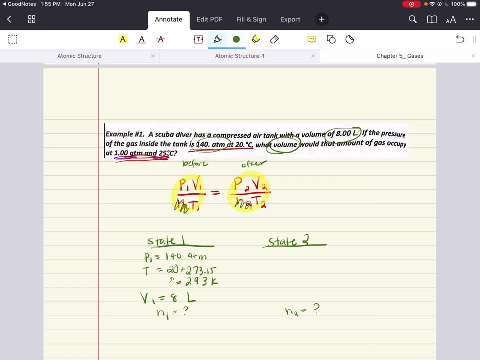 If you're not sure, you can look at state two, and you can look at state two and you can look at state two. So you can kind of just omit N1 and N2.. Since they're not given to you, they're. 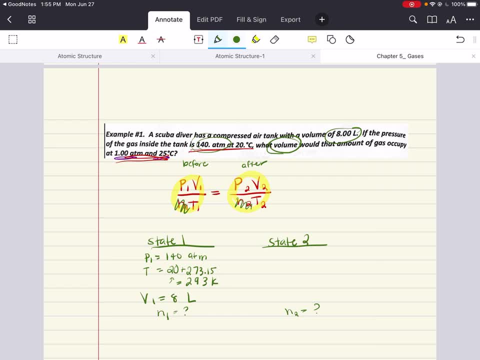 assumed to stay constant. And if they stay constant, there's no need to introduce them into our equation. Fantastic. Now for state two. we're working under one atmosphere. We want our state two to be at one ATM. all right, The temperature is at 25 degrees Celsius. 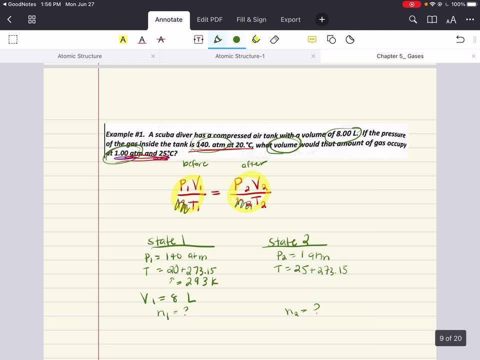 but we want it in Kelvin. So 25 plus 273.15, that's like 298 about Kelvin, all right, And we are trying to figure out what the temperature is. So we're working under one atmosphere and we're. 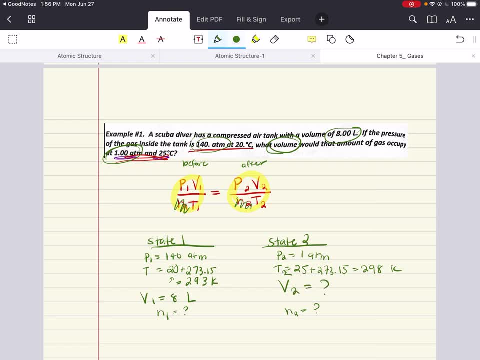 trying to figure out V2,. what is the new volume? all right, So we're solving for V2,. all right. So sometimes these word problems can be confusing because you don't know what state to associate these variables to. all right, But we can read it again now that we've assigned it and see that if 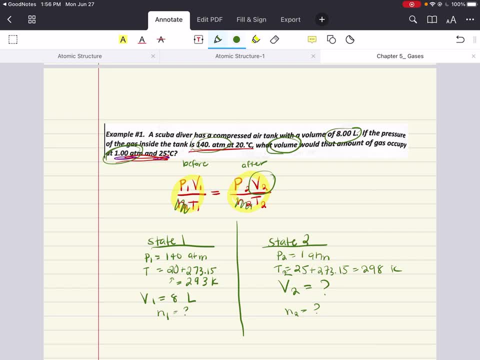 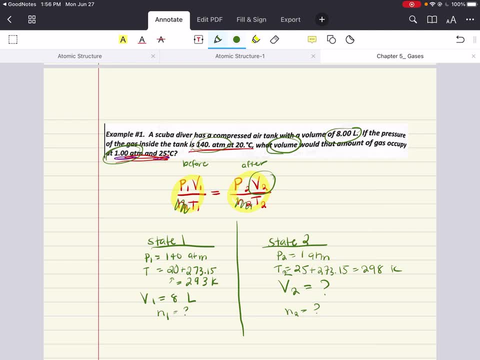 that eight liters- that's what they're talking about- is 140 ATM at 20 degrees Celsius. all right, Those are all our initial conditions of state one. What volume would that amount of gas occupy, though, if you change the conditions of pressure and temperature? That's essentially what the 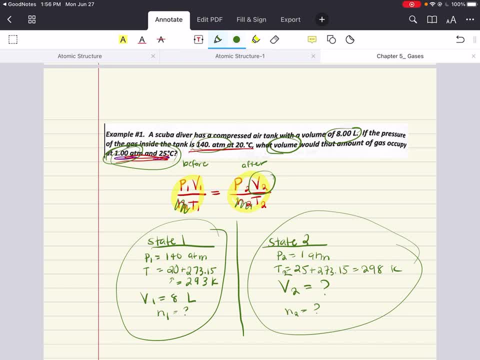 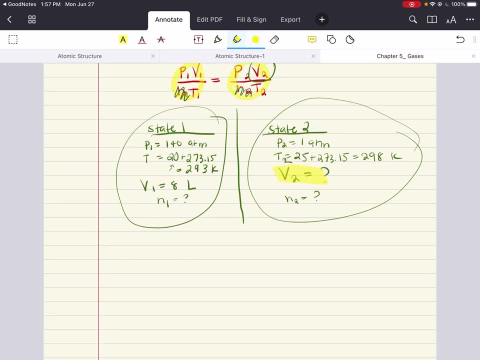 problem is saying: and that's how we were able to identify state one from state two and figure out what variable exactly we're trying to figure out, and that's V2.. So now that we know we're trying to solve for V2, this becomes a very easy problem. We're just going to move variables, all right. 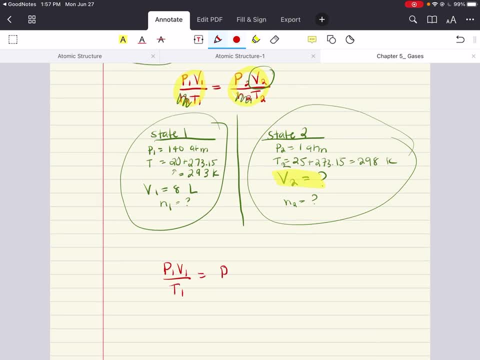 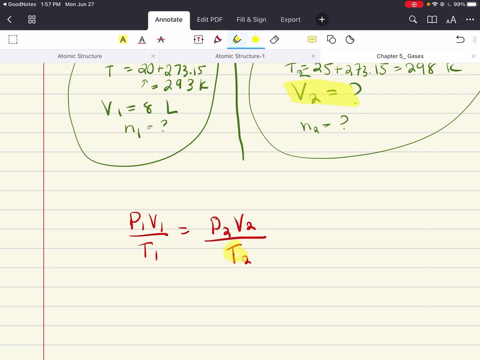 We're just going to move variables so we can solve for V2,, all right. And how we're going to do that is well, first we're going to move temperature over. Okay, we're going to multiply both sides by T2 to cancel out T2 on this side, all right. And then we're going to divide by P2 on both sides, as 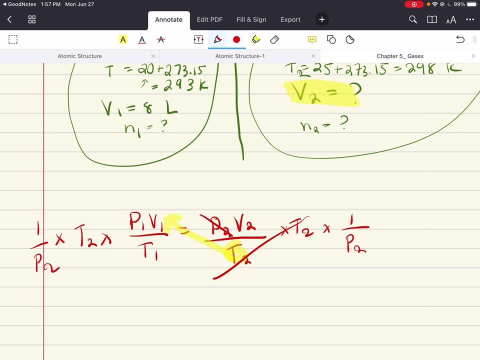 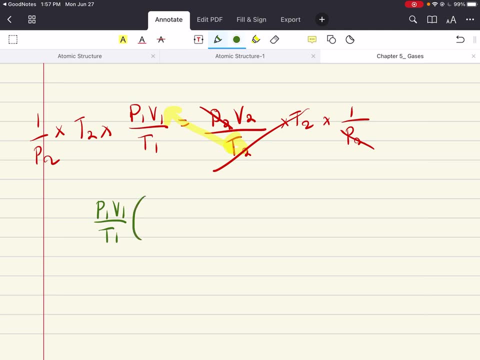 well, so that on this side P2 is given. So we're going to divide by P2 on both sides as well, so that on this side P2 is given, It gets canceled as well. So what we have now is an expression of P1V1 over T1, all right times T2. 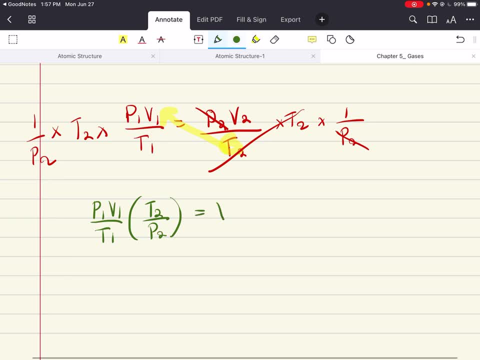 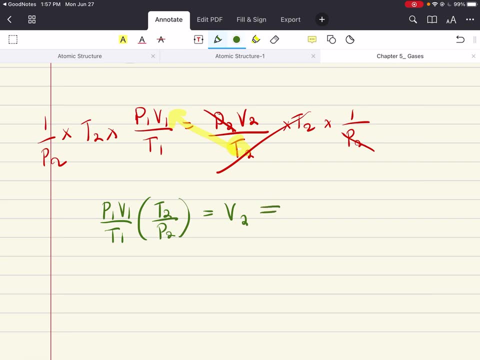 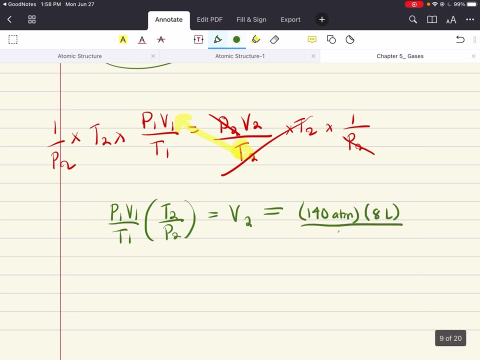 over P2 is equal to V2, all right. So that's our new expression: Plug in everything. all right, Let's plug in everything. That's: 140 atm for P1, all right. 8 liters, 293 kelvin, all right. And 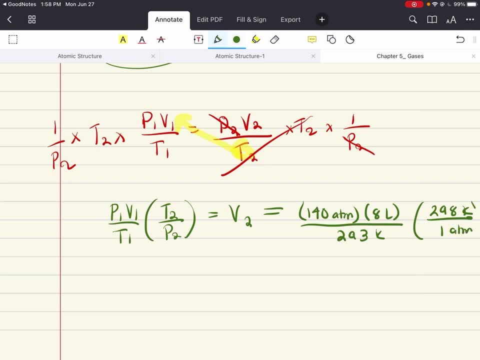 what's our new expression? 298 kelvin, over 1 atm. all right, We're just plugging in all the variables. Plug it into a calculator. What you're going to get is 1.14 times 10 to the 3 liters. 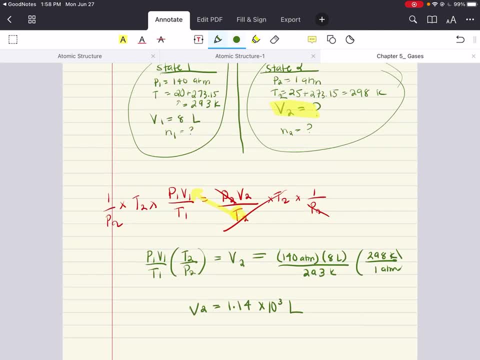 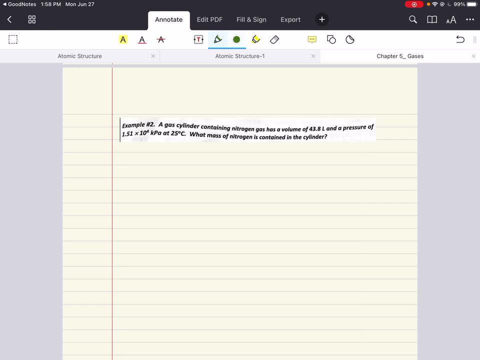 and that's it. That's how you solve this problem, all right. So for the second one, I want you to attempt it. Same sort of concepts, all right: Ideal gas law and combined gas laws. Take advantage of that and attempt to answer this question. Let me know what you get in the 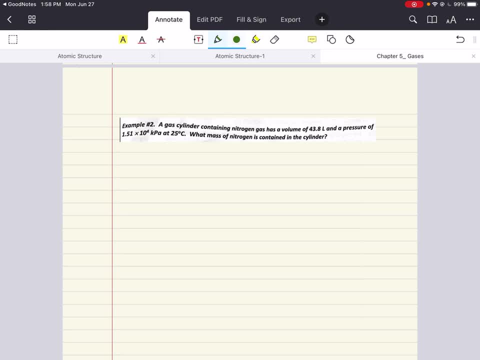 comments below and I'll let you know if you got it right or if we need to rework it together. All right, awesome, Let's do this third one together, All right? 55 grams of a certain gas occupies 10 liters under STP conditions. Remember STP conditions, standard temperature and pressure. 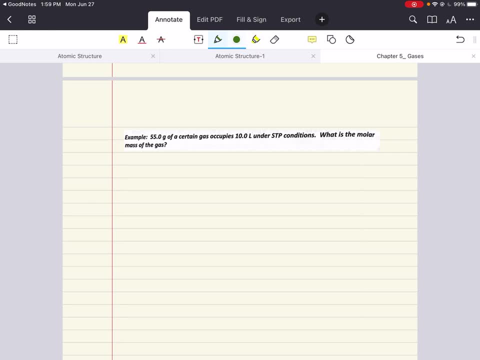 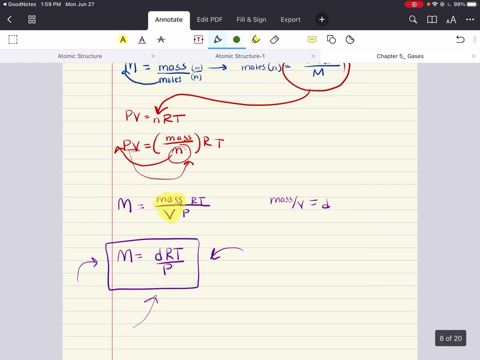 means that we're operating under 1 atm and 273 Kelvin. All right, it's asking: what is the molar mass of the gas? All right, so you know how we derived this equation that relates molar mass to variables like density, temperature and pressure. Well, we're going to take advantage. 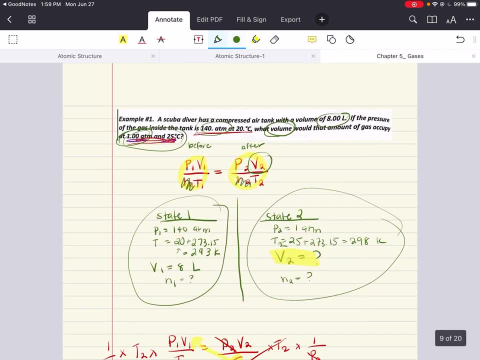 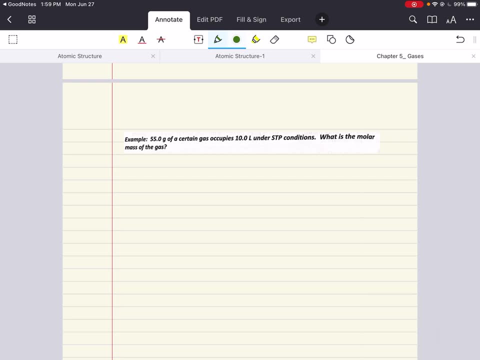 of this relationship that we derived here to answer this kind of problem. Because, just looking at the problem, all right, we know what kind of variables we have to work with. All right, we're going to write down everything we know and we're going to see that. 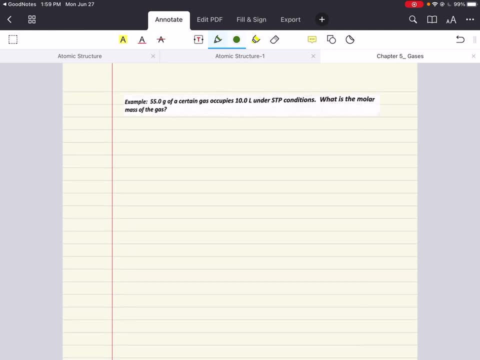 that relationship is going to be the most useful for us. All right, what kind of things do we know? Well, we know the mass. We're given 55.0 grams of a gas. All right, we have the liter, we have the. 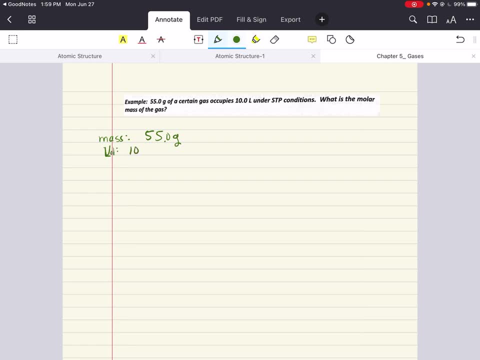 volume: Volume: All right, it's 10 liters, All right. we know we're operating under standard temperature and pressure, which means we know that the pressure is 1 atm and we know that the temperature is 273 Kelvin- All right. So if we look at our definition of molar mass, 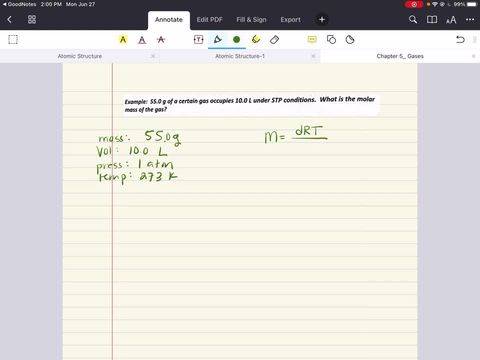 as density times gas, constant times, temperature over P, or in other words, mass over volume. for density, all right, times RTP. what we realize, all right, this is what we derived earlier. What we realize is we have all the variables we need to solve this problem. It's just plug and chug. 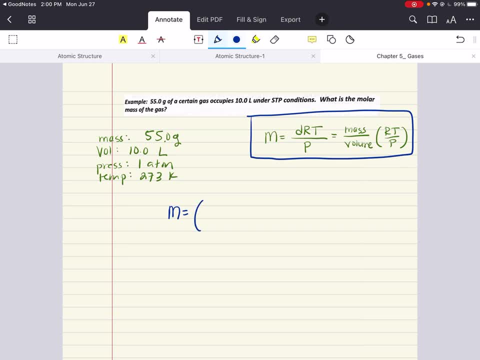 All right. So molar mass is equal to mass, 55 grams over volume. 10 liters, All right, Fantastic, Very easy, All right Times. gas constant. The gas constant is, we'll rewrite it, 0.08206 liters atmosphere over mole dot Kelvin. 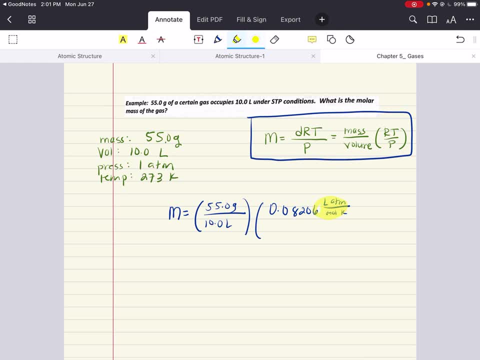 I know I wrote the gas constant for you earlier. but looking at the units for this gas constant, all right, you realize why. for volume, we only operate in liters. for pressure we only operate in atm moles and Kelvin is because we want to make sure that when we plug everything into our 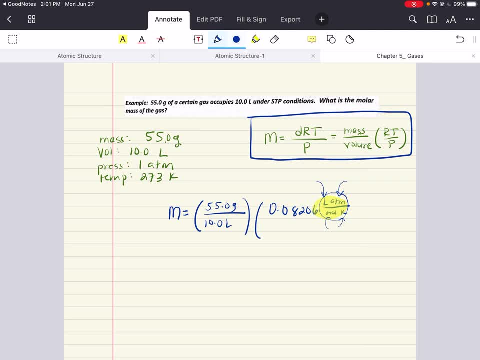 ideal gas law or combined gas law, Or this definition of molar mass that everything cancels out, which is why we always make sure that we're not putting in Celsius, we're putting in Kelvin, so that Kelvins can cancel out and we 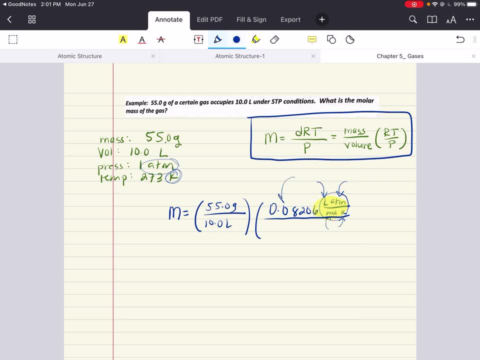 can obtain the unit we want at the end. All right, So if you're using this particular gas law, this is the unit associated with that. So you want to make sure all your other variables match these units for volume, pressure, moles and temperature. All right, Just a heads up. 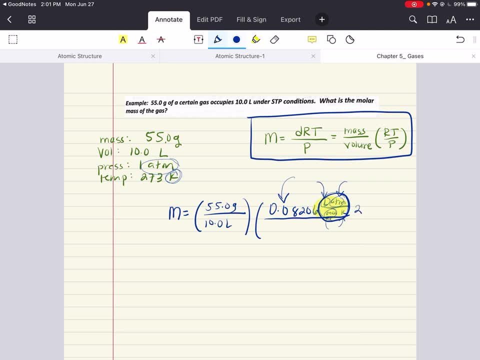 just an FYI: All right Times, 273 Kelvin. all right over pressure, 100 atm. Put this in a calculator and what you're going to get is 123 grams per mole. That's the molar mass of the gas. Fantastic, This next one.